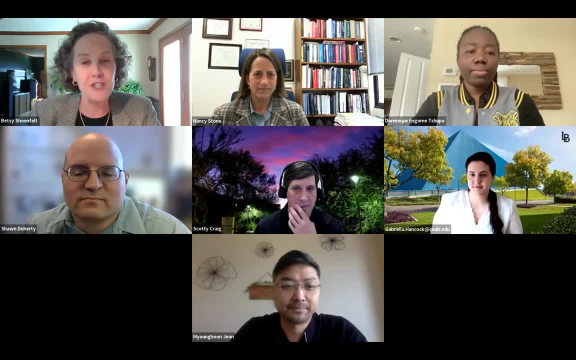 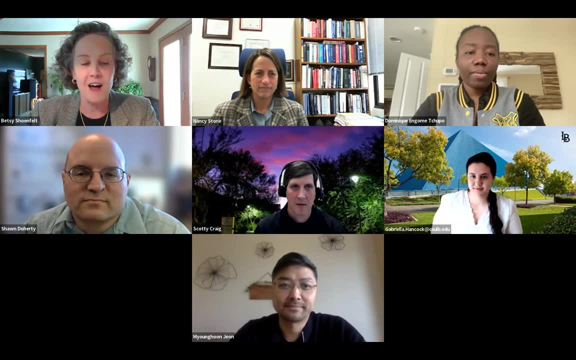 This session is being recorded. Hello and welcome to the American Psychological Association series on careers in applied psychology. I'm Dr Betsy Schoenfeld, a university distinguished professor, emerita and industrial organizational psychologist at Western Kentucky University. I'm representing the APA Office of Applied Psychology and I will be hosting this panel. 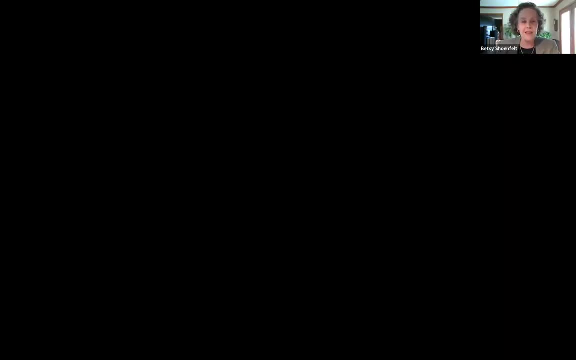 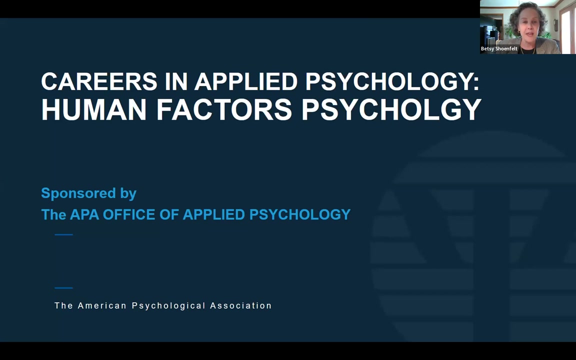 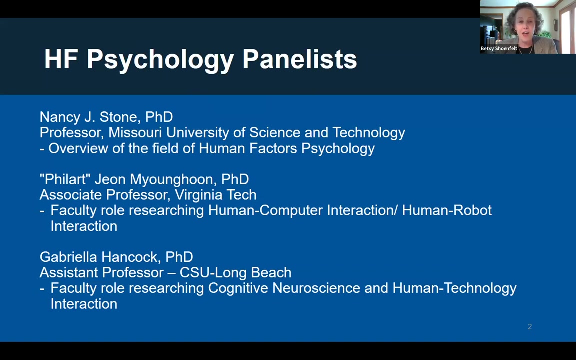 Today we have a very interesting and informative panel on careers in human factors psychology. We have six panelists who will describe different career paths and human factors. First we have Dr Nancy Stone, professor at Missouri University of Science and Technology, who will provide an overview of the field of human factor psychology. 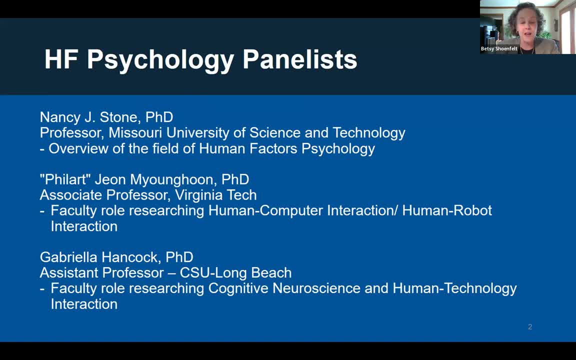 I will also mention that Nancy is the current president of APA Division 21,- Applied Experimental and Experimental Psychology. Next we have Dr Philip Myung-hoon, who is associate professor at Virginia Tech. He will speak on his role with computer interaction and human-robot interaction. 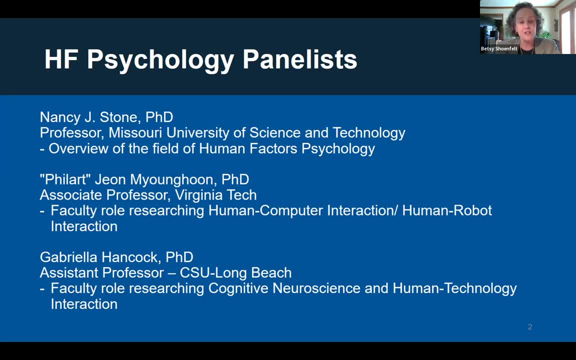 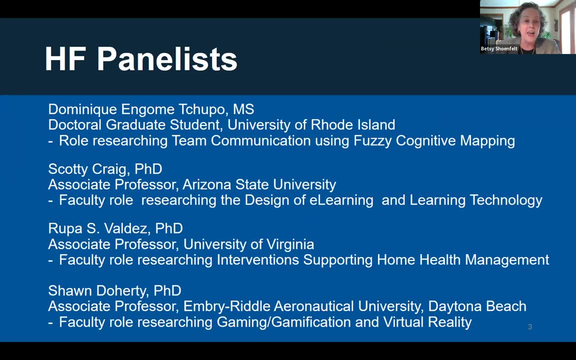 Next, Dr Gabriella Hancock, assistant professor at CSU Long Beach, will share her role researching cognitive neuroscience and human technology interaction. Next, Dominique Ignomi-Chupo, a doctoral graduate student at the University of Rhode Island, will share her role researching team communication using fuzzy cognitive mapping. 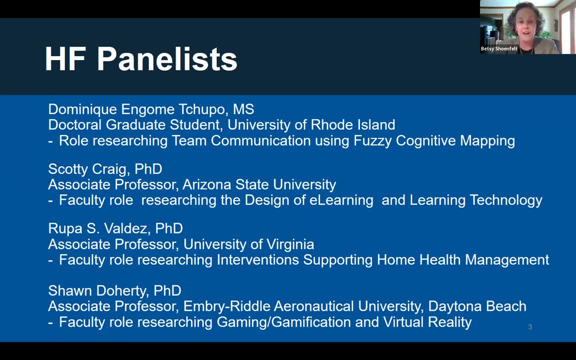 Next, Dr Scotty Craig, associate professor at Arizona State University, will share his faculty role researching the design of e-learning and learning technology. Dr Rupert Valdez, who is associate professor at the University of Virginia, will describe her role researching interventions supporting home health management. 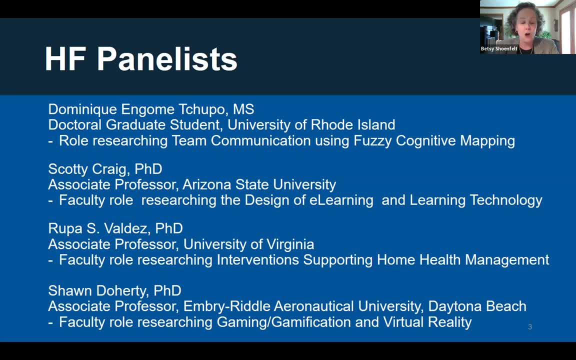 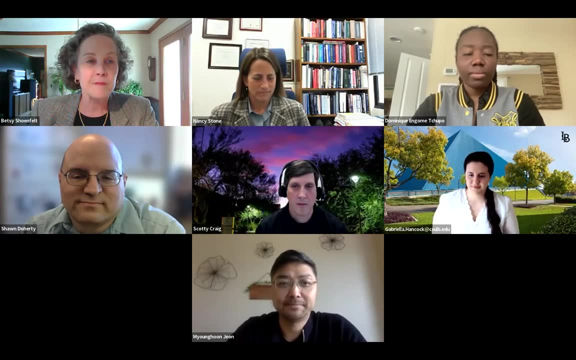 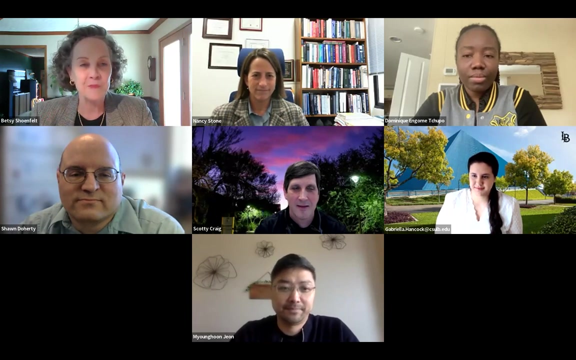 And finally, wrapping up, Dr Sean Daughtry, associate professor at Emory-Riddle Aeronautical University, Daytona Beach, will describe his faculty role researching gaming, gamification and virtual reality. Now Nancy will start us off with an overview of the field of human factors. Thank you, Nancy. 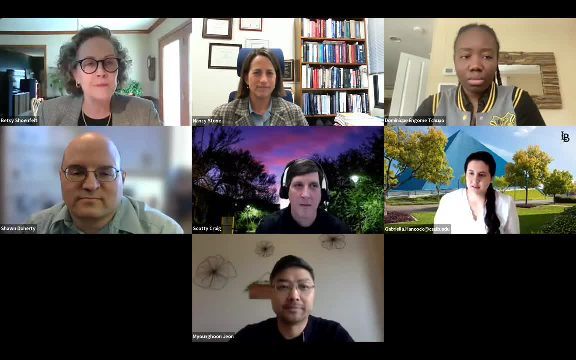 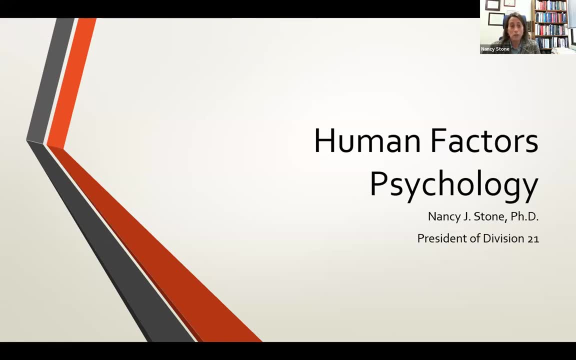 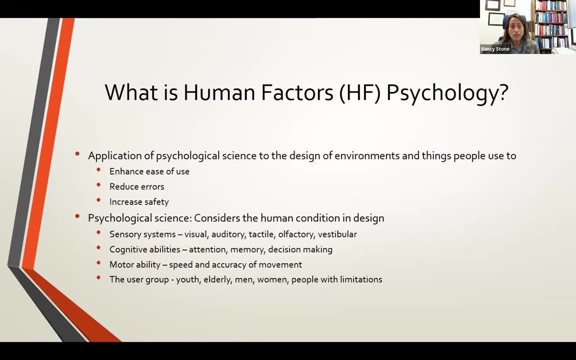 Stop, I can't. Well, thank you, Betsy, and thank you for the opportunity to give an overview of human factors psychology as president of Division 21.. So human factors psychology can be described as the process of taking psychological science and using that knowledge to design environments and things people use. 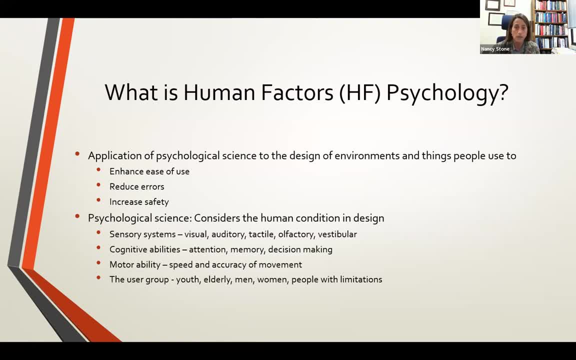 What we're trying to do is to make the use easier for people, which can help reduce errors and increase safety. sometimes, So, when we're talking about psychological science, we're considering the conditions of the human and we're trying to apply that to design. 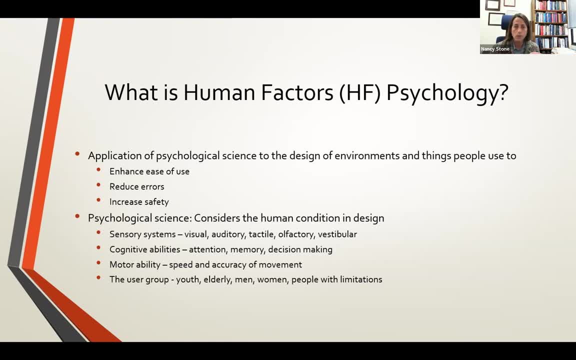 So we're concerned with sensory systems: How do people see, How do people hear? We also are concerned with cognitive abilities: How much attention is needed for a particular activity? What kind of memory is going to be needed, or decision making, to be able to use the environment or the things that we're designing for them? 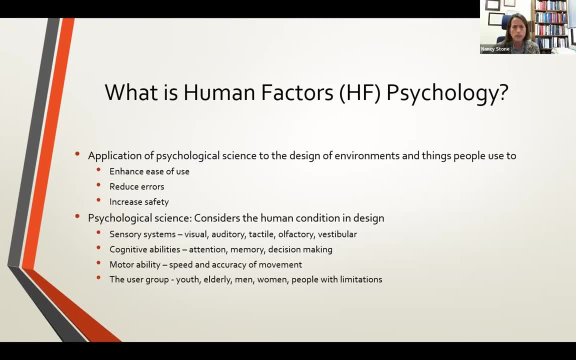 What about motor ability? Do people have to move their fingers or their arms, their legs? What's the speed of movement and how accurate will they be? But we also have to be really cognizant of the user group. Are we designing an educational system for young children or for the older adult? 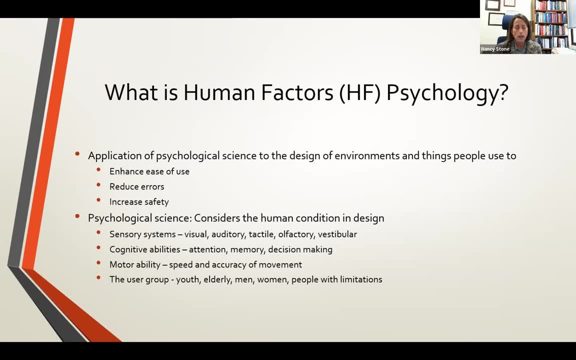 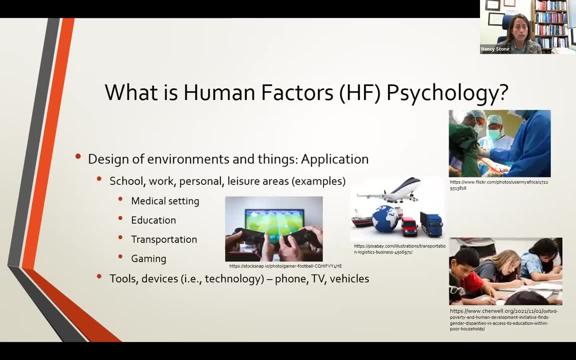 Or are we designing it for people with limitations? How do we design this so that it makes it easier for people to use? Now, the environments is when we take and apply the psychological science. So the environments could be a variety of things. It could be at school, it could be at work, it could be in your personal space. 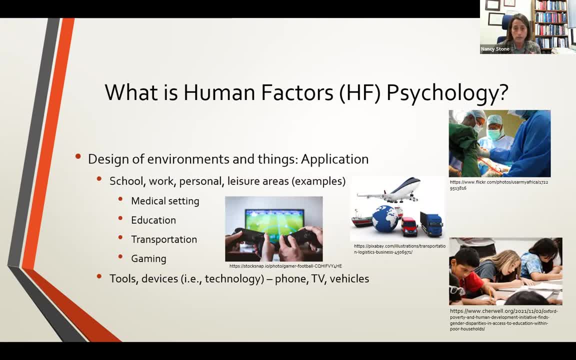 So, just to give you some examples, we have the health situation or medical settings. If you're in an operating room or an emergency room, how do we design that environment and the tools that they use so that they are more efficient and more effective? 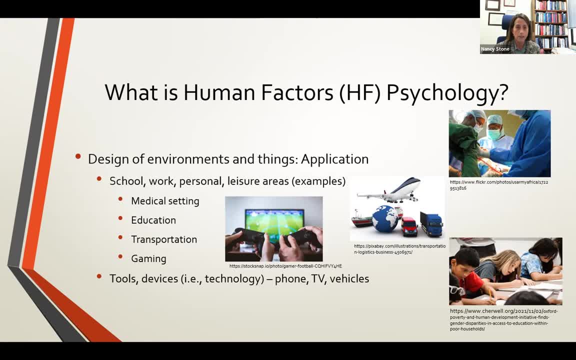 And, of course, there's greater safety. The person in that situation is going to be in a much better situation. You can also think about education, So is the educational material designed well for people to learn and use? What about the environment, in the sense of lighting, or the chairs or the tables that they use? 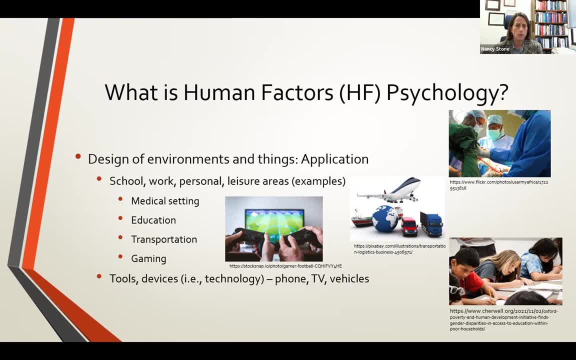 And also we can look at transportation. We often talk about aviation Because we want to make sure the planes fly well and safely, But we also are concerned with the transportation of our own vehicles. So, for instance, you get into your own car. 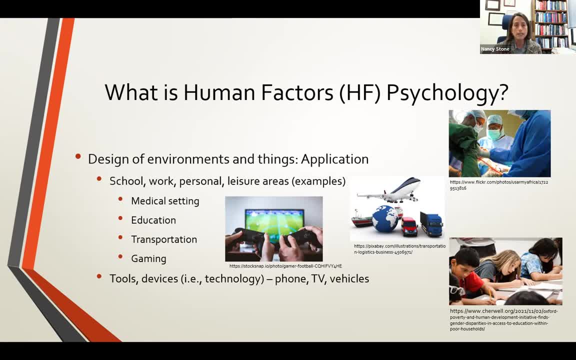 Are the things within that car easily understood so that you can use it and be safe, not only for yourself but other drivers on the road? Plus, now, with artificial intelligence coming in, how does that play a role in influencing the transportation safety and ease of use? 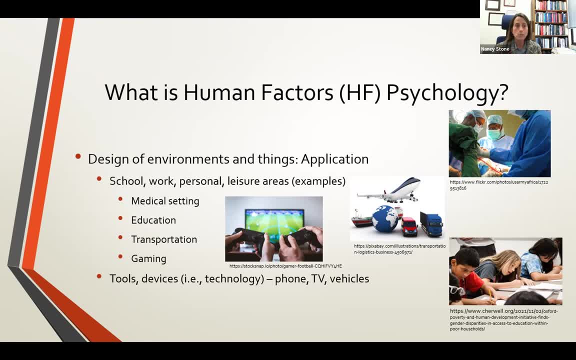 But we can also apply human factors to gaming. How do we design a game so that it's intriguing and challenging for a user, but they also understand how to use it? So this includes a lot of the tools or devices. So you might be trying to design your phone or a TV, or the vehicle. 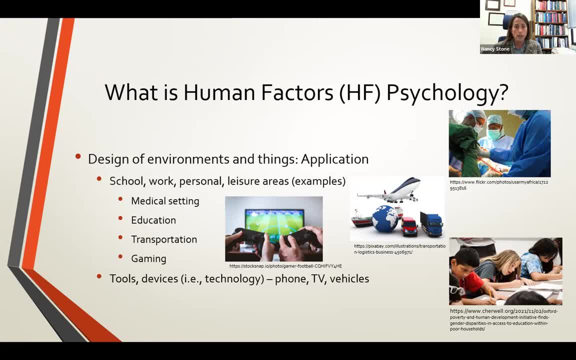 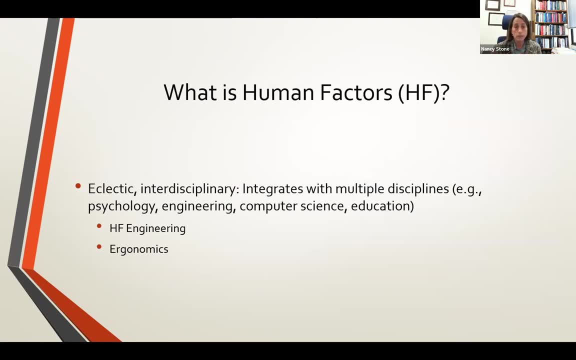 So there's a lot of different tools or devices that we might need to design as well. So human factors as a discipline is eclectic, It's interdisciplinary, It pulls from multiple disciplines. We have psychology, We have engineering, We have computer science. 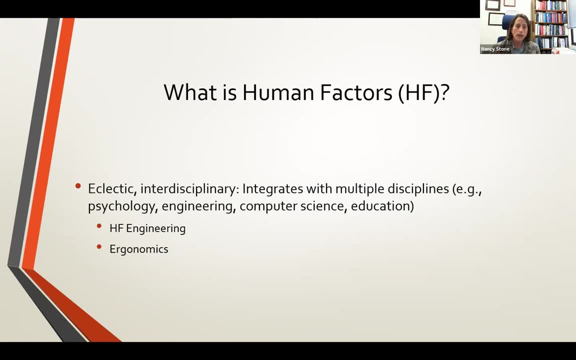 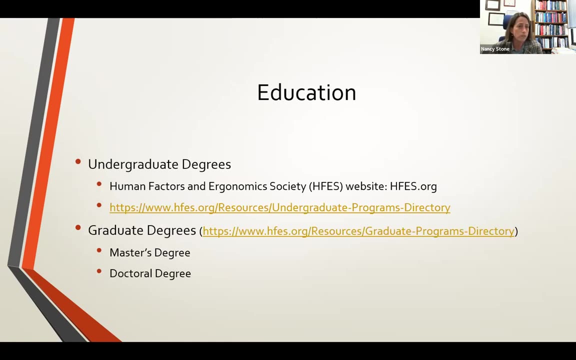 And you can throw in a number of other disciplines as well. So there's human factors engineers as well, And there are ergonomists also, who learn and apply psychological science and the engineering into design of things people use. If you're interested in gaining an education in human factors, 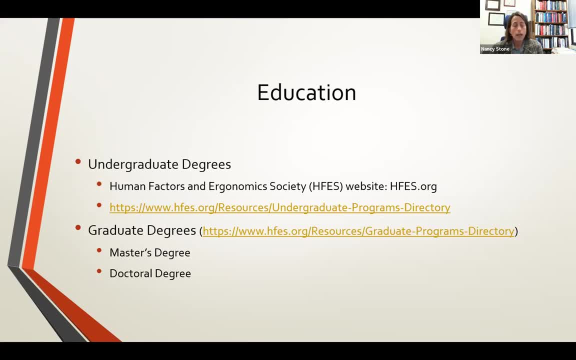 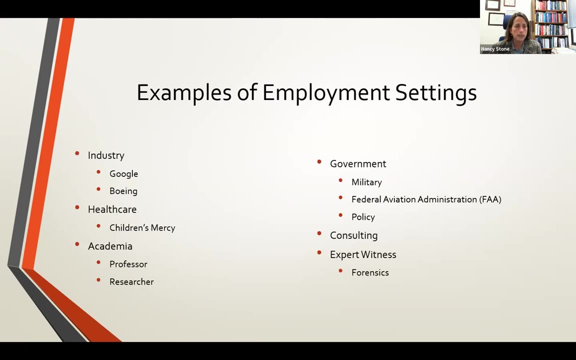 I've given the human factors and ergonomics website And they do have some undergraduate degrees and they have a listing for that. But they also have listings for graduate programs, the master's level and doctoral degree. Just some examples of employment settings. 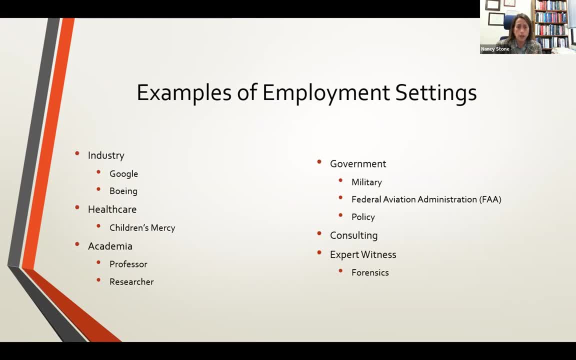 There's industry And there's, of course, healthcare, And a number of hospitals are hiring human factors specialists. You can work as an academic or be a university professor. You can teach and do research. Some people work in government, So they work with the military in designing things that are safer and more easily used. 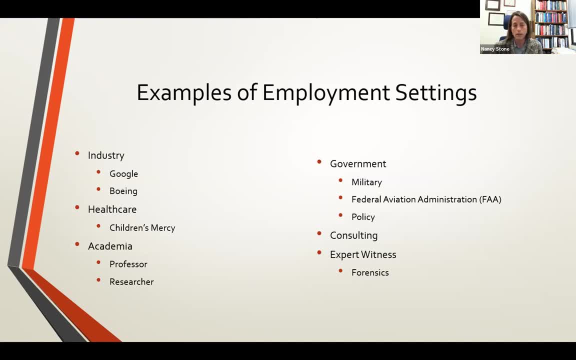 Or even creating policy to ensure that things that are being designed are following a proper process. Others are in consulting. They have their own consulting practices, Or some people are expert witnesses. So when things don't go quite as well as we would like or somebody gets injured, 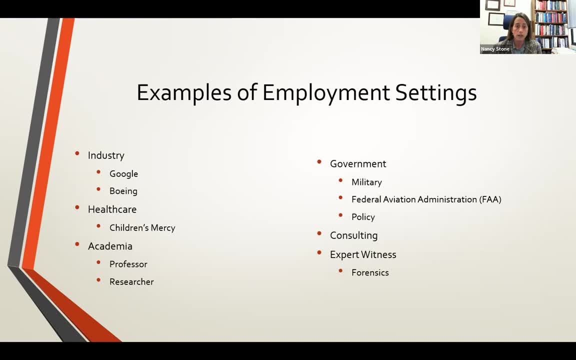 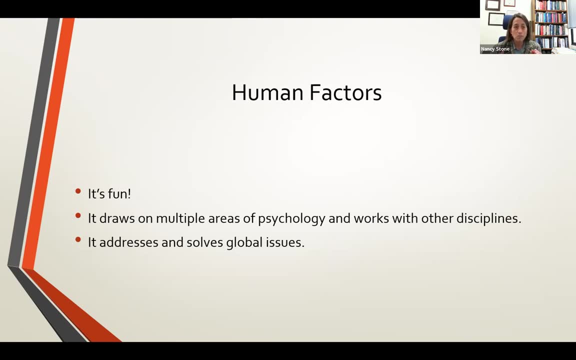 they might bring in somebody to explain why it didn't function as well. So, in a nutshell, what I would say is: human factors is really fun. It draws on multiple areas of psychology And it works with other disciplines, And it addresses and solves global issues. 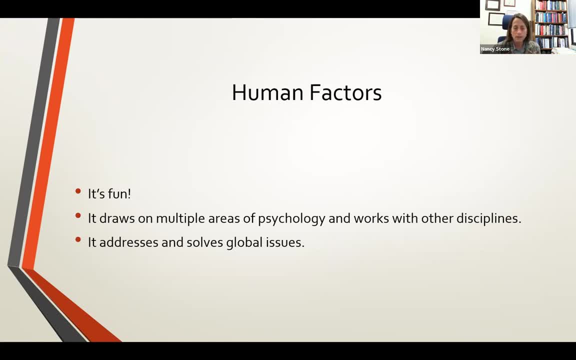 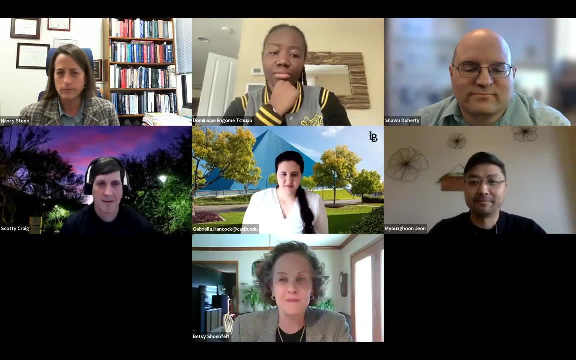 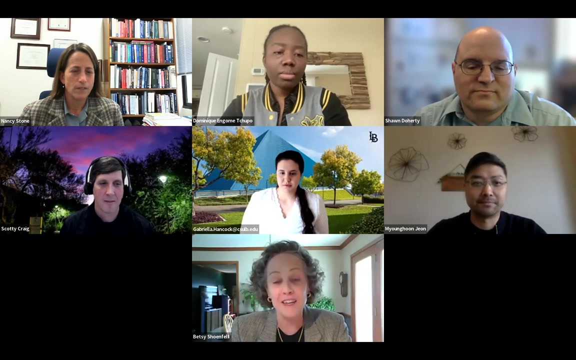 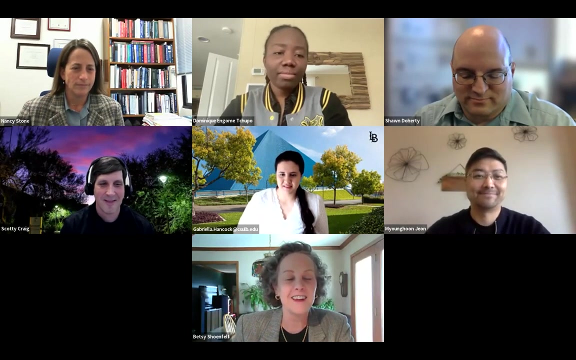 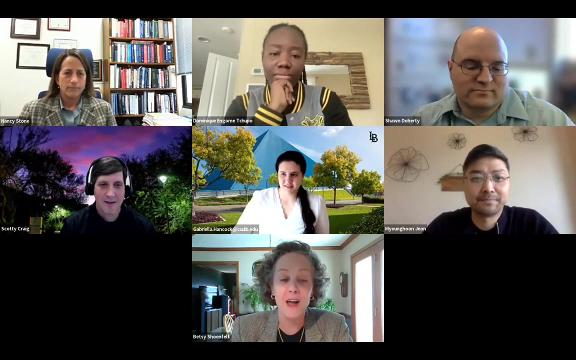 So with that I'll turn it back to our host And I look forward to hearing what the other panelists have to say. Thank you, You're muted. Thank you, Nancy, for that overview of human factor psychology. Hopefully this has piqued interest to hear from other human factor psychologists about their careers. 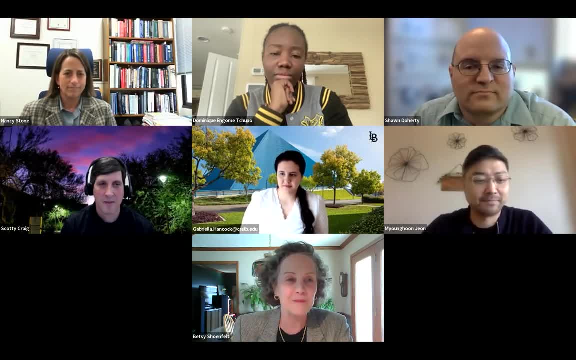 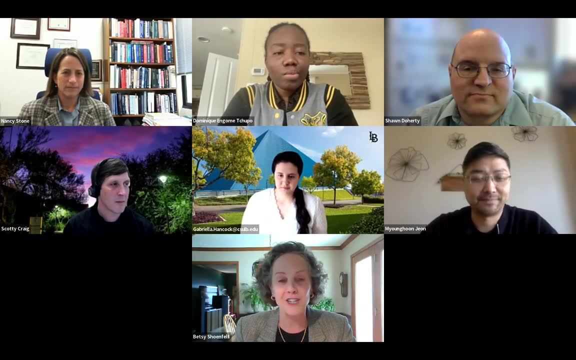 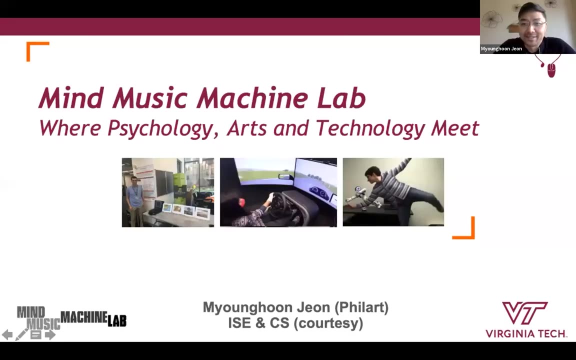 And our panelists are prepared to do just that. Next, Phil Art will be presenting his presentation. Next, Phil Art will speak on human-computer interaction and human-robot interaction. Okay, Thank you, Betsy. My name is Myunghoon Jeon. 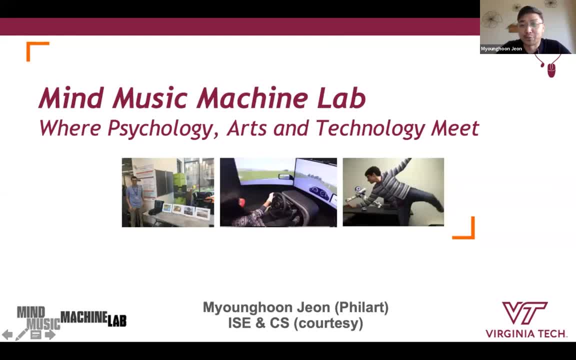 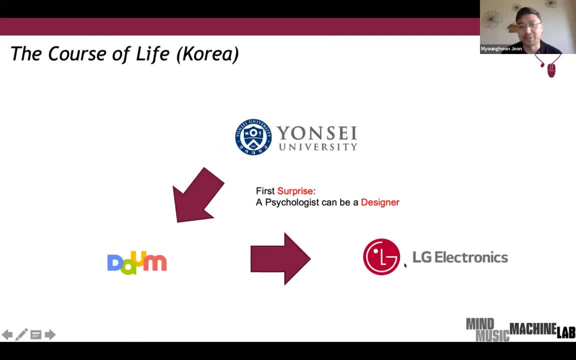 You can call me Phil Art, which means love art. I'm associate professor in the Department of Industrial Systems Engineering and Computer Science at Virginia Tech, So my journey in engineering psychology started when I was a college student at Yonsei University in South Korea. 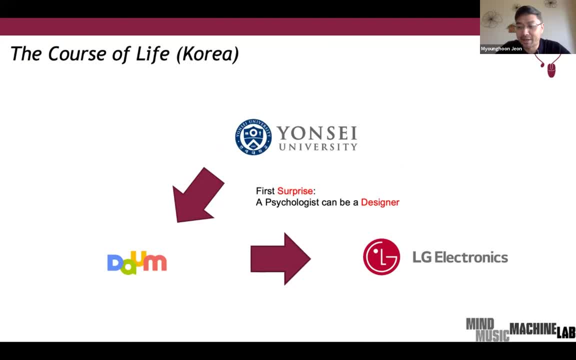 So when I was sophomore, I took a course that's about psychology and modern society. That was a team teaching course And one of the faculty members introduced psychology and design. So whoa, I didn't expect that. So I wanted to dig into that more. 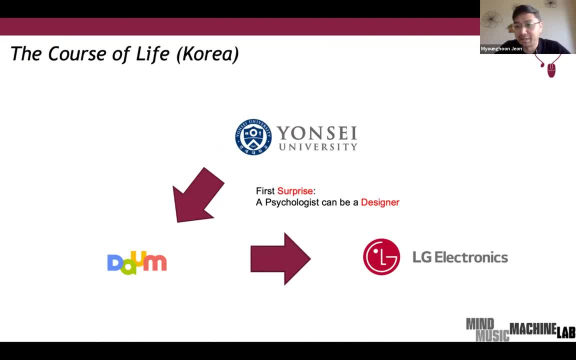 And I went to graduate school master's program called cognitive science, But my specialty was in engineering psychology. So after I got my master's degree I went to industry. So my first job was at Daum Communications. That is kind of Google in Korean version. 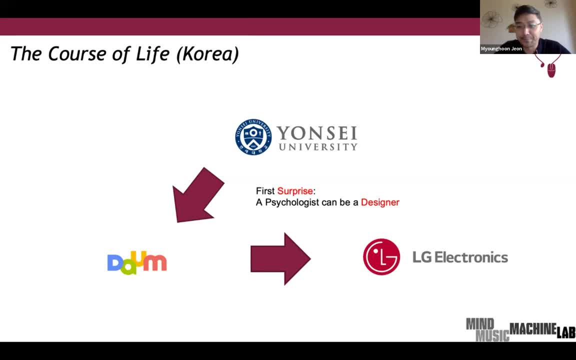 So I worked there as human-computer interaction researcher And then I moved on to LG Electronics and worked there as a user experience designer. So the first surprise: So if you do research in engineering psychology, then a psychologist can be a designer. So while I'm doing work in an industry, 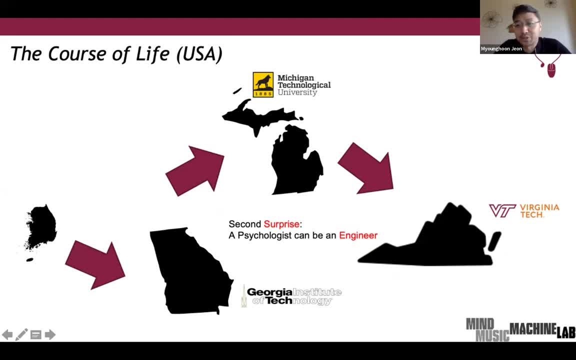 I thought I probably need to study more in my domain. So I went to Georgia Tech And studied there engineering psychology and got my degree- PhD degree- in engineering psychology and human-computer interaction. Then I got my first academic job at Michigan Tech. 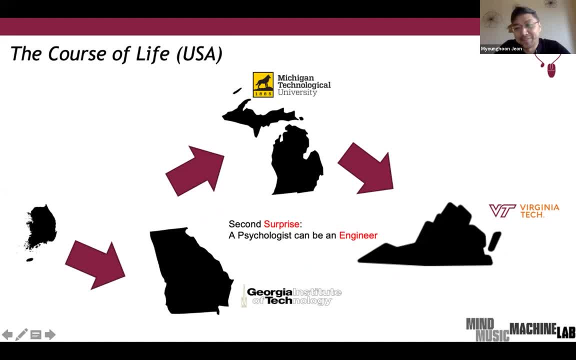 So I went to North Up And I worked in two departments as joint professor- So human factors program and computer interaction And computer science program- And both departments were under college of sciences and arts. So I'm still in science and arts. And then in 2018, I moved to move back to South. 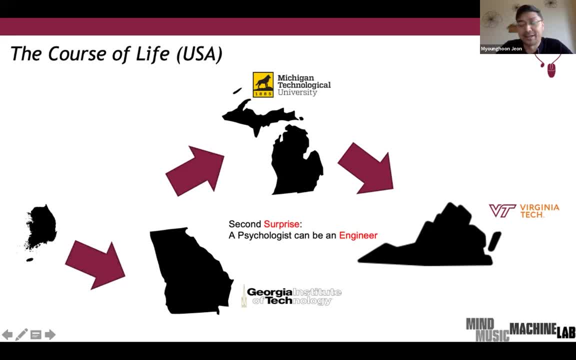 So at Virginia Tech, where I am right now. So I am working at industrial systems engineering, which is under the college of engineering. So you know what? I started in humanities, Went to sciences and arts And then now I'm working at engineering department. 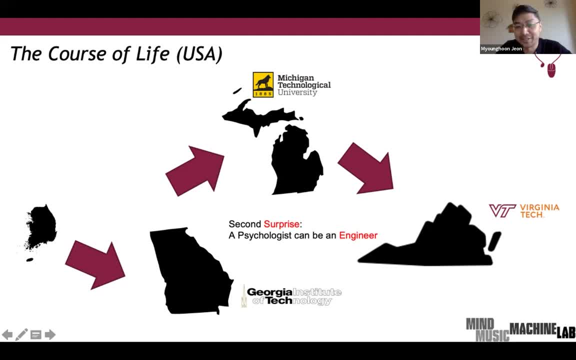 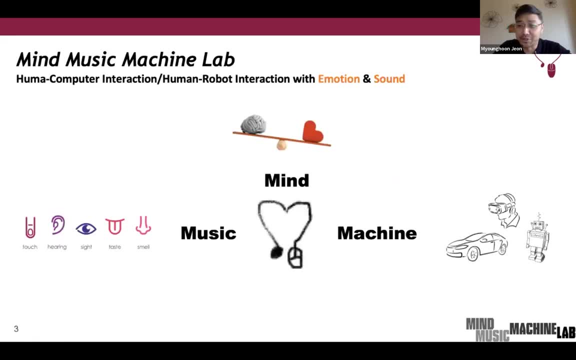 So second fun fact: If you study engineering psychology, then psychologist can be an engineer. So my lab is called mind music machine lab And we do research on human-computer interaction and human-robot interaction, And I have two research themes. 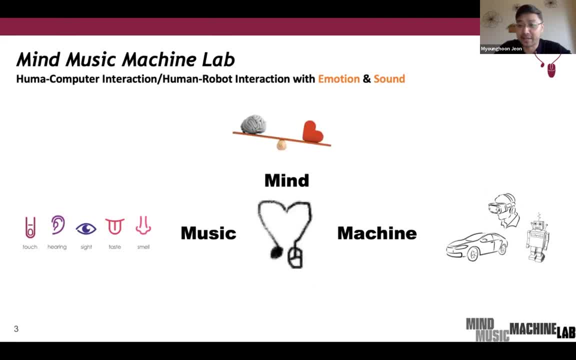 Emotions and sound. So to better design the interactions between people and technologies, We need to understand holistically the human mind right First. So traditional human factors research- they really has focused on cognitive processes. We use an analogy: of information processing. 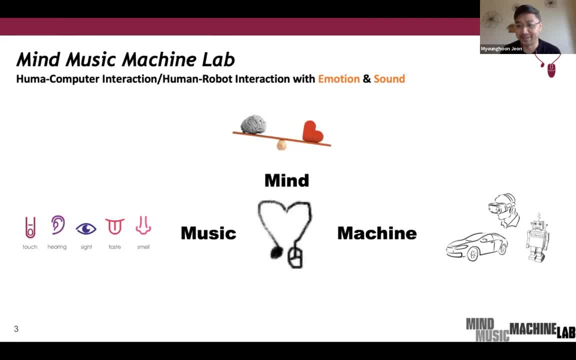 But we all know we also have emotions and affect right. So that's why we do research on emotions as well as cognition in my lab, And then, likewise, traditional human factors research. They do research on visual interface And graphic user interfaces. 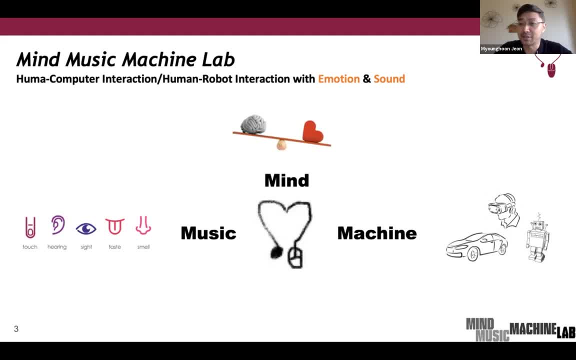 But, like I said, we want to do holistic approach. So we do research on audio, sound and multimodal displays. So that's why my lab is called mind, music and machine. So I have three different research application domains which include three different machinery. 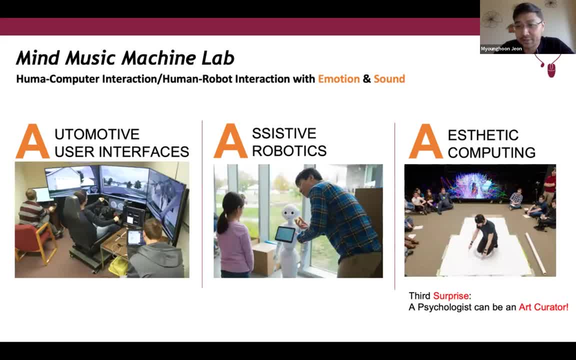 So the first is automotive user interfaces. So nowadays we do a lot of research on automated vehicles, So in data, Different levels of automation, How drivers can develop trust, How emotions influence that procedure And how we can design sound in order to display. 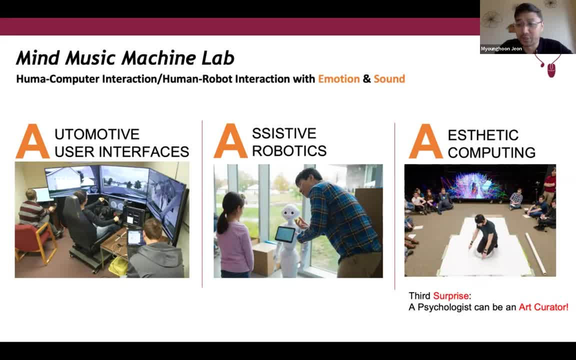 And we do research on assistive robotics. So we do design new robots for kids with autism And we also do research with kids in school settings to promote STEM education. And, the last but not least, we do research on aesthetic computing in immersive environments. 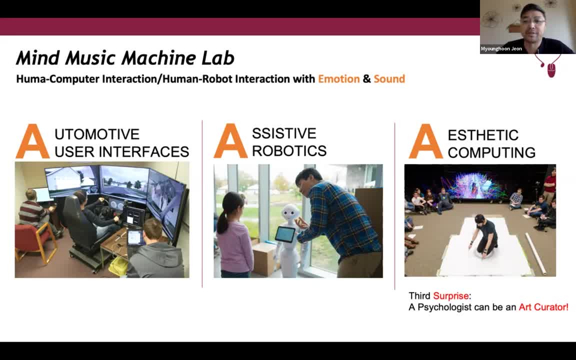 So in my lab we do research with performing artists- dancers, musicians and visual artists- So using all kinds of technologies we have- So we have multiple displays and motion tracking sensors and robots- And how musicians and performing artists, they utilize all these technologies and create new experiences and art. 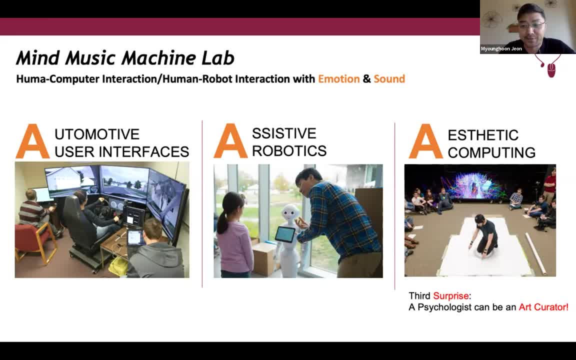 That's what we're doing, And we frequently do performance in the lab. So the third fun fact is here: If you do engineering psych, maybe sometime you can be an art curator, which I'm doing. So that is kind of fun fact. 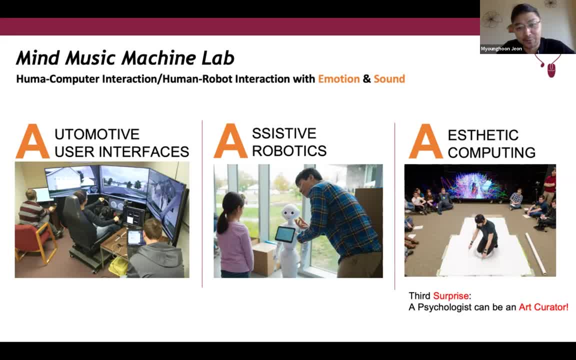 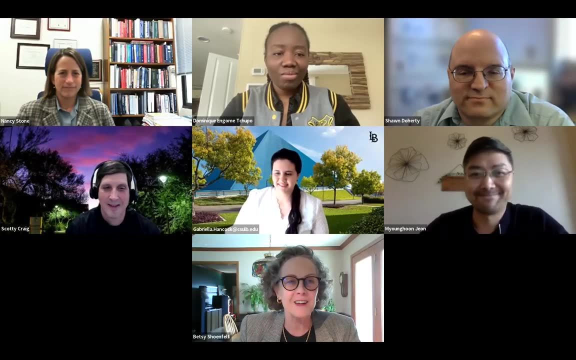 So I want to stop here, And I sincerely hope that all these presentations today can help you make an informed decision about your future career as a psychologist. Thank you. Thank you, Philip, That was quite interesting. Next we have Gabby speaking on cognitive neurodiversity. 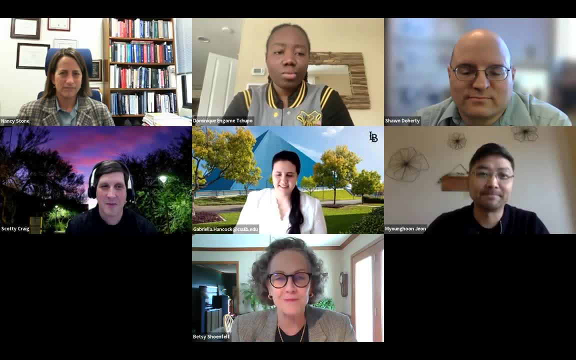 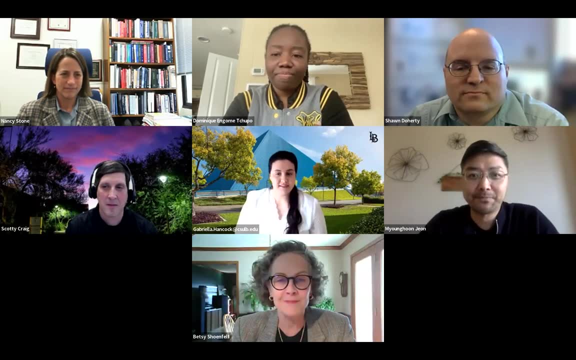 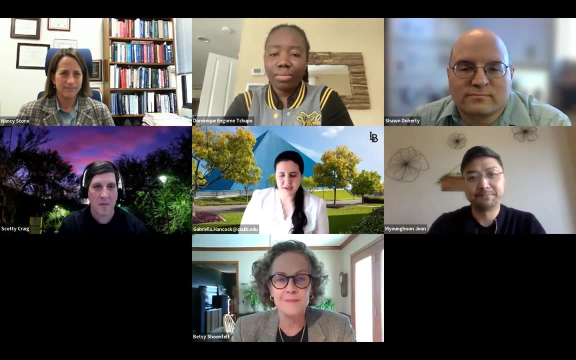 And she's working on cognitive neuroscience and human technology interaction. Hello everyone, Thank you so much for having me. So I'm Gabriella Hincock, assistant professor at California State University, Long Beach, and the director of the Stress and Technology Applied Research Laboratory. 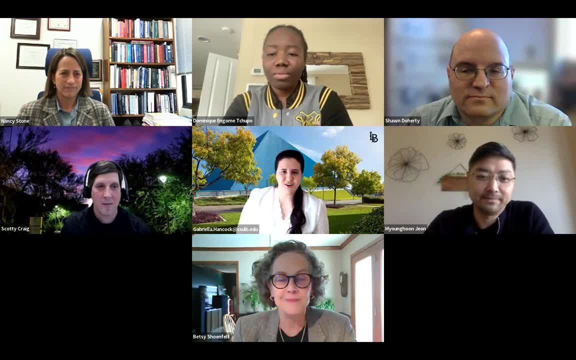 So kind of getting my start in this area. I always like to say that I'm nobody's example for this, Because I got the one-two combination of nature and nurture. I had a parent in human factors, a professor of human factors, which is incredibly rare. 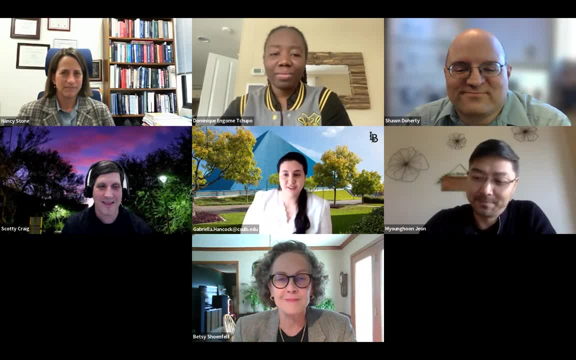 And I also had a parent who was a professor of early childhood education. So I got a love of teaching and research And I got all of those dominant genes because my sister is in none of it. So that's how I ended up here. 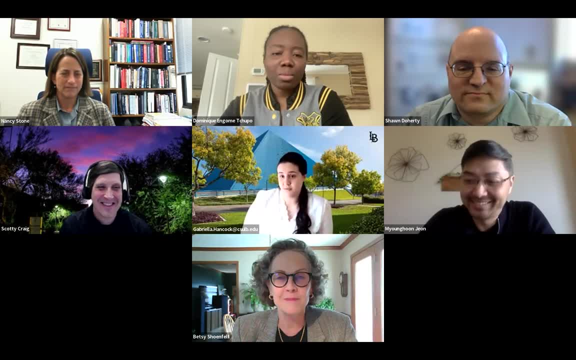 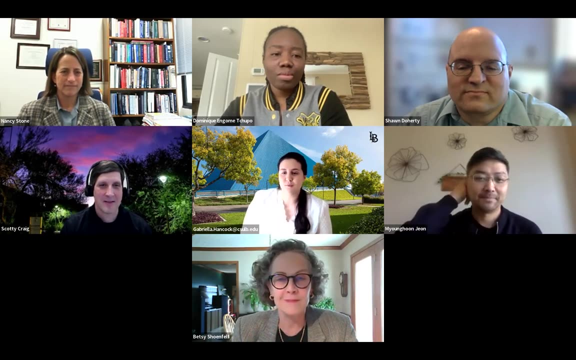 So I had the luxury of knowing what I wanted to do, which I realize is not everybody's path along here. But one of the things that got me interested in human factors, and has kept me interested in human factors all of this time, is that anywhere there is a human doing anything, we apply. 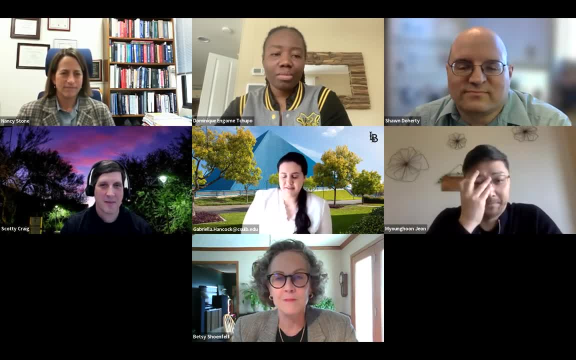 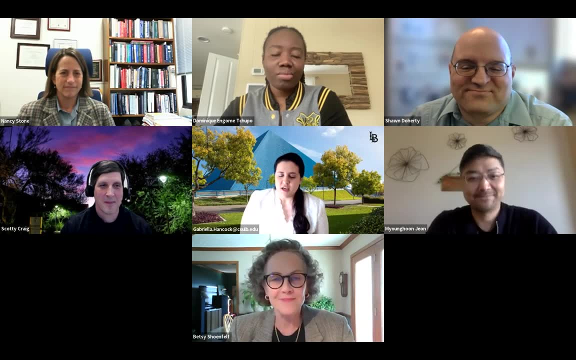 So the sky is the limit And anything that I'm interested in. I have free reign to study, So that's why I'm here And that's why I will stay here. So a little bit about my background. that got me to that point is I have a bachelor's degree in psychology. 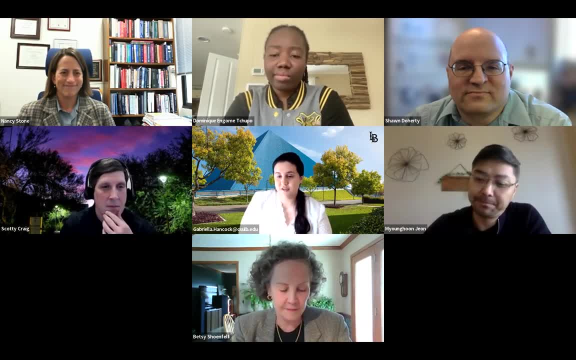 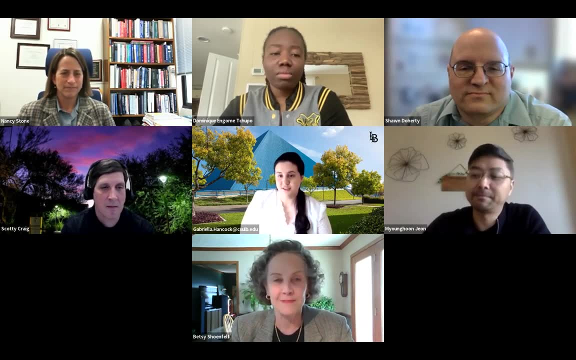 A master's degree in applied psychology And a master's degree in applied psychology, And I have a PhD in applied physiology and kinesiology, Another master's degree in industrial engineering And a PhD in applied experimental and human factors psychology, And without an understanding of that field, that seems like a really eclectic hodgepodge of what is it that you do? 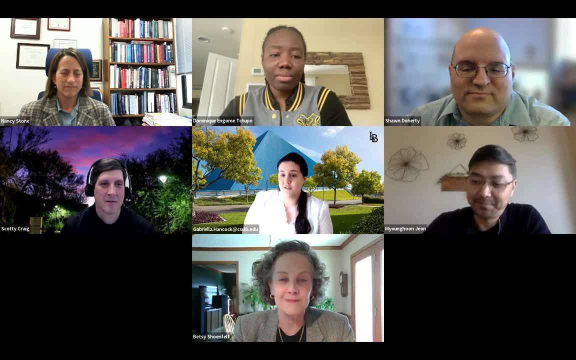 But, like Dr Stone pointed out, human factors thrives on that kind of multidisciplinary input. So there's actually method to the madness, Because, right, psychology is all about how the mind works. Physiology and kinesiology is all about how the body works and how it produces performance. 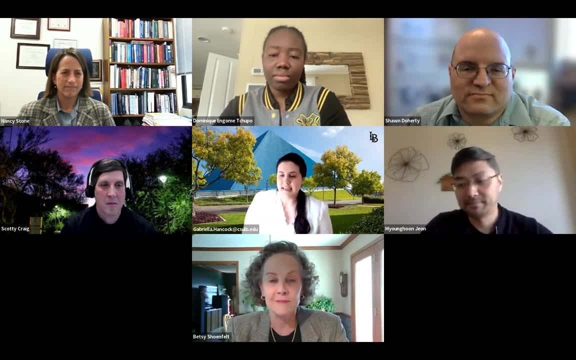 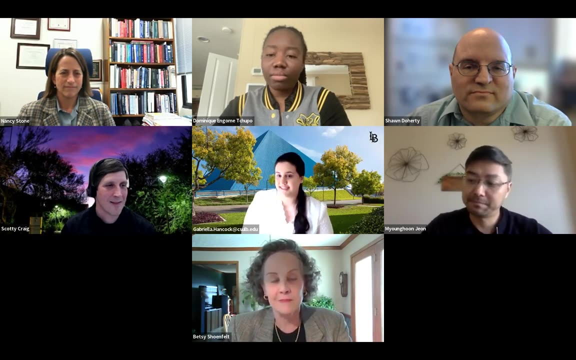 Industrial engineering is all about large-scale human machine systems And then applied experimental and human factors. psychology ties that all together, About how mind, body and the environment and the system come together to produce those outcomes of effectiveness, efficiency, safety and fun that we try to maximize in our field. 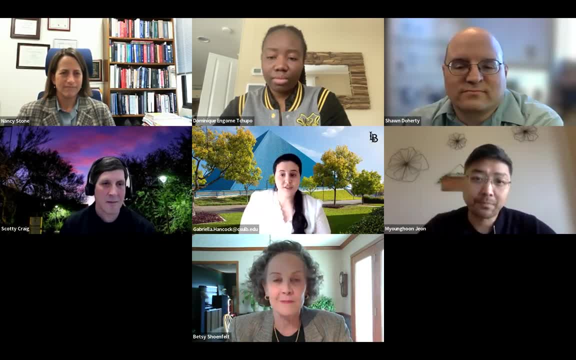 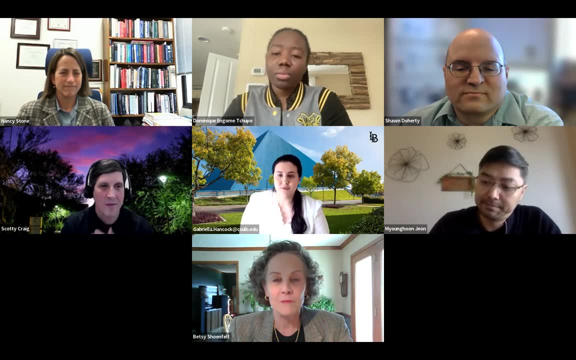 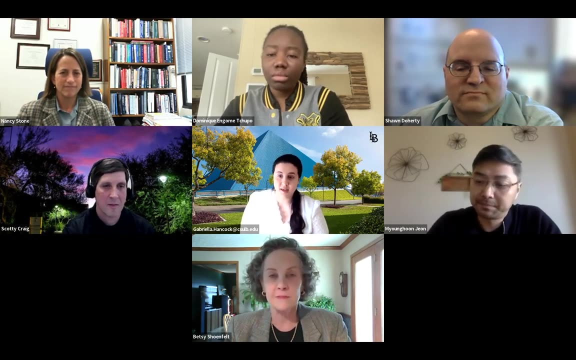 So, as a university professor, my career has really three main thrusts: Teaching, which I absolutely love, And I am very lucky in that the courses that I teach are human factors focused. I teach intro, I teach methods, I teach a seminar on human-computer interaction. 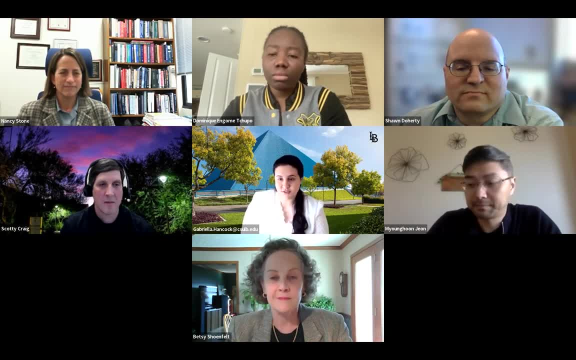 The second thrust is service, which revolves around student development and helping the field through peer review editing, Organizing conferences and so on and so forth. But the majority of what I wanted to talk to you about today is the third branch, which is research. 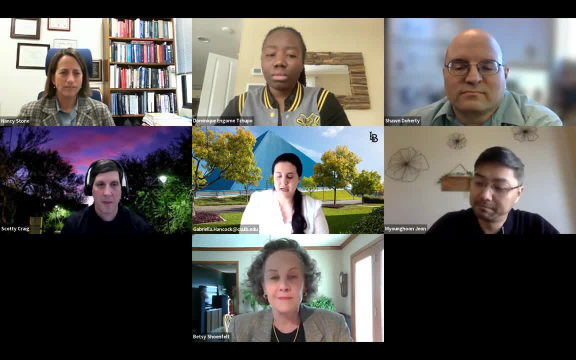 And, as Dr Schoenfeld pointed out, in that mix of different disciplines that I told you about, my specialization is using cognitive neuroscience methods and measures to understand that relationship. So if we want to design systems to help people prevent and improve their mental health, 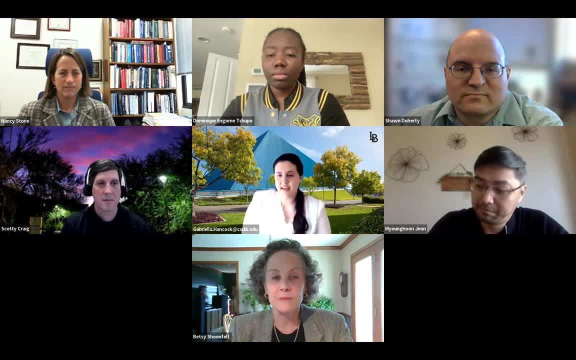 If we want to design systems to help people prevent or help prevent, pardon me, things like fatalities, injuries, accidents, property damage, you know, all of these horrible outcomes that we don't want to have- We have to establish where it is where human performance goes wrong, right? 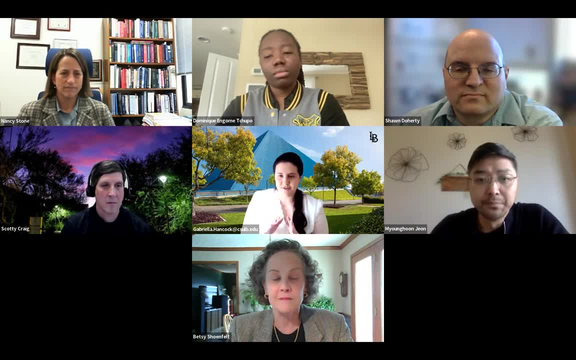 So where is that kind of cusp of catastrophe And how can technology help to pull people back from that front? And part of things, a couple of different ways that you can do that. You can do that through performance, But in some of the systems that we use performance goes so quickly that you might not get an opportunity to see that something is going to go wrong until it already has. 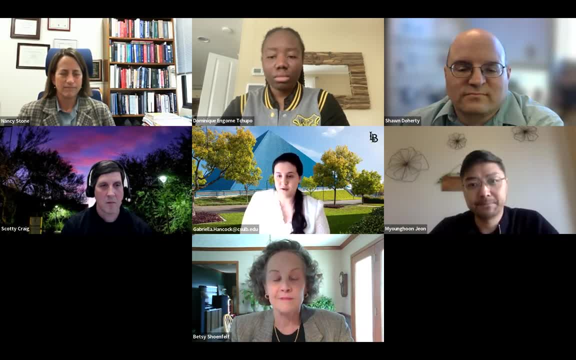 So that's not really going to help us predict super well. Another option is through self-report measures. So questionnaires, right, How stressed are you? But the thing about those perceptions is that they are just that perceptions, So people might not recognize how stressed they are right. 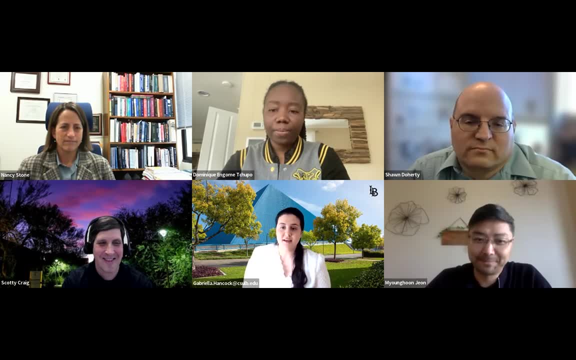 They might not have the ability to, They might not have the ability to understand what is influencing their performance themselves. Also, you know, people can lie, So we can't take those to be as reliable an indicator. But the thing about the body is that the body doesn't lie right. 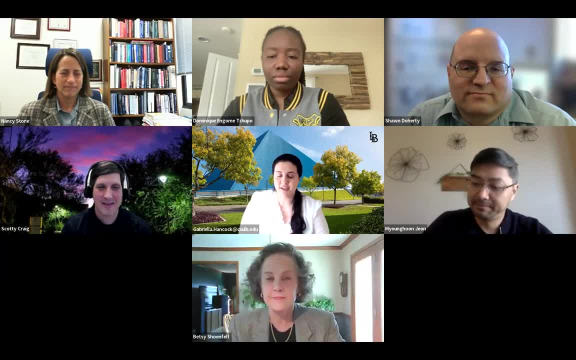 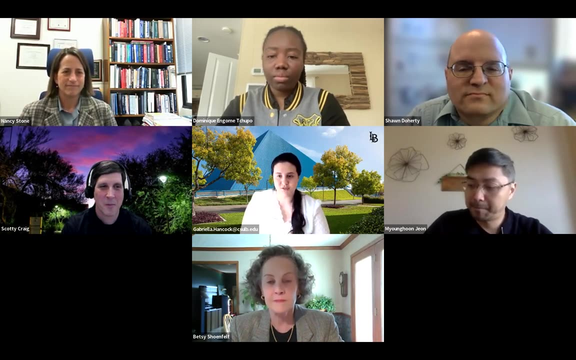 Your heart can't tell you it's not beating for a particular reason. So that's one of the reasons that I love it. It's continuous assessment, so you can do it throughout performance And it's very interesting. It's very interesting to see how all of the systems of your body come together to produce that performance. 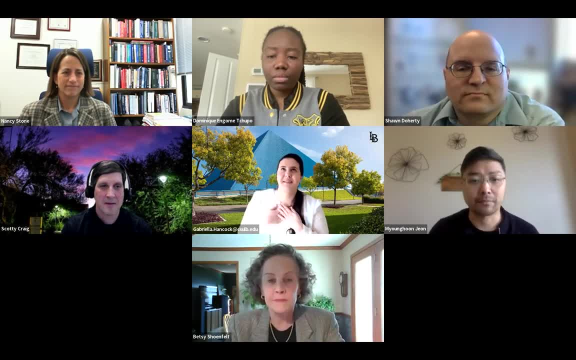 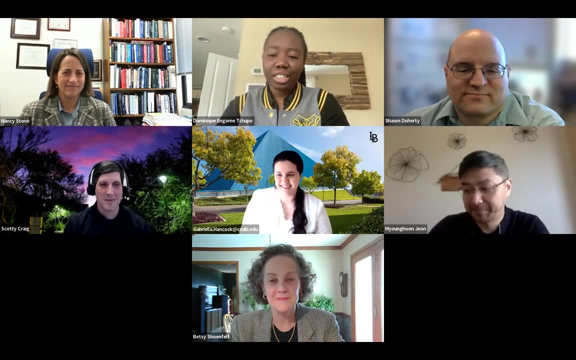 So I have specialized in the past with the brain. The brain is my first love. The heart, the muscles, skin conductance response. I've got a little bit of sweaty palms right now as I'm nervous presenting to you because I understand all of the physiological mechanisms doesn't make it, doesn't protect against that kind of stress. 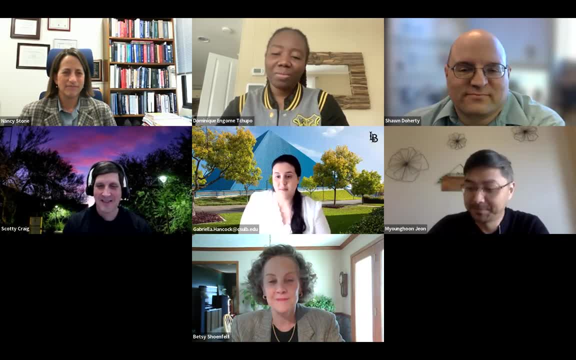 So I wanted to talk a little bit about some of that work that I've done. So, as an applied neuroscientist, some of the work that I've done in the past has been with the US Army, So prior to our our exit from that area of the world, when our troops were deployed, the number one threat to their life and safety were improvised explosive devices. 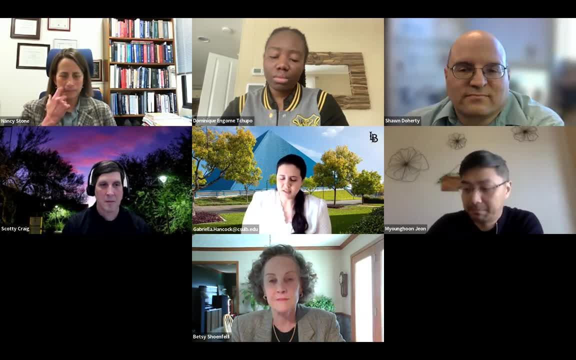 So those are things like roadside bombs. So the problem is: So the problem is right. it's like looking for a needle in a haystack which is inherently hard, but you also have certain parties who are trying to make that needle look more like the hay. 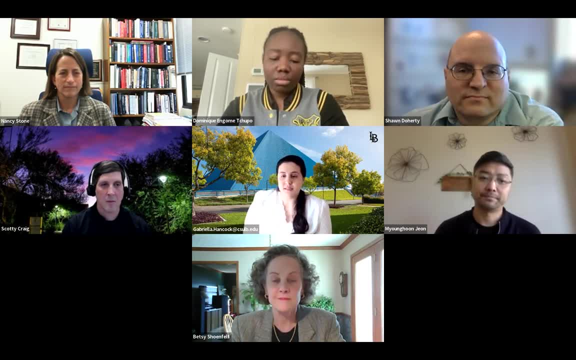 Right, So, and so the big problem is that these soldiers know what it is, that they're looking for it, they know exactly what to look for, But the thing is that the human brain is not wired to pay attention for hours at a time. right, even if it is to save your own life. 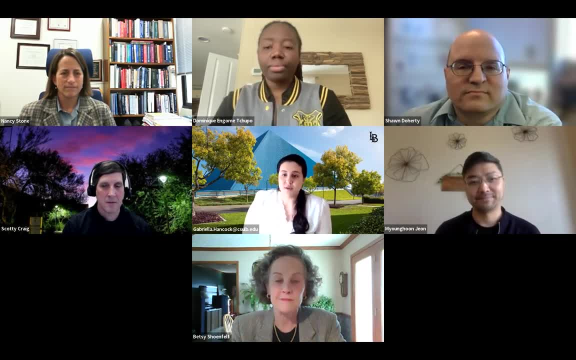 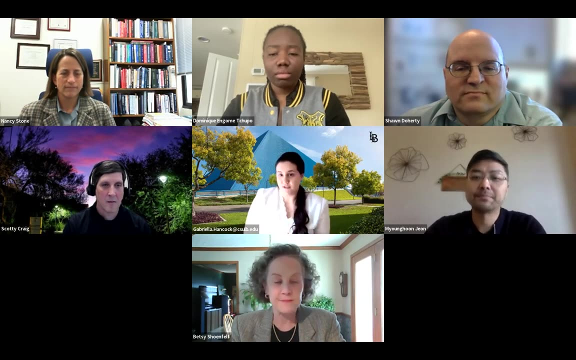 or the life of your team members, And so what I was doing was looking at cerebral oxygenation of the frontal lobe, which is right here behind your forehead, and it is the area of your brain that is responsible for decision making, Right? So is that a threat to me, yes or no, Right? Is it not a threat? what should I do now? And so I was looking at those changes in the brain and how I could you help to use those to predict, not when there is or is not a signal, but whether or not. 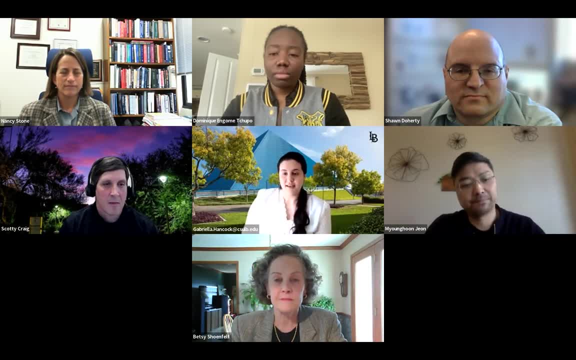 the person was more or less likely to miss it Right. so the brain is more likely to miss it because they weren't paying attention. And if they can, if we can track that, the computer can then say: hey, you know, I've noticed that for the past minute or so you've kind of not been paying attention to the tasks, so it would. 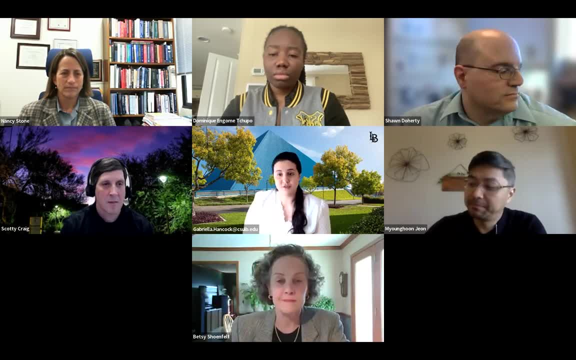 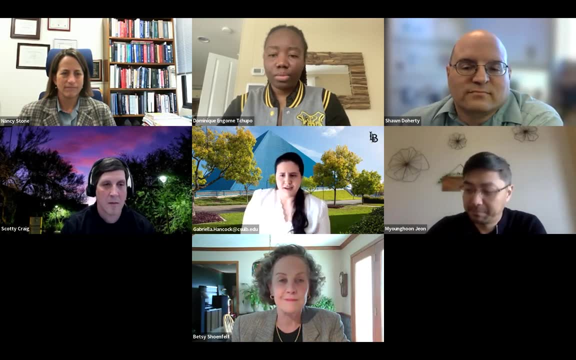 really help if you could reorient yourself. So that's one example of applied neuroscience and how to enhance user experience and safety. I'm user COVID, Excellent. So that's my one example of applied neuroscience. So that's my one example of applied neuroscience. 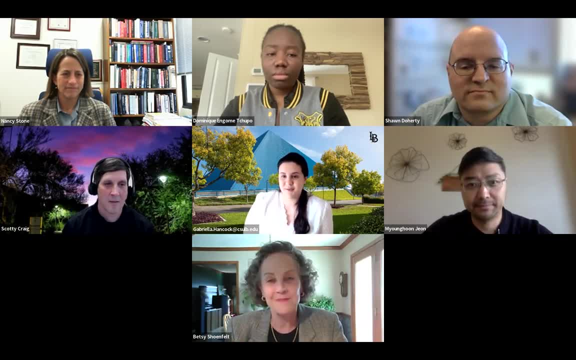 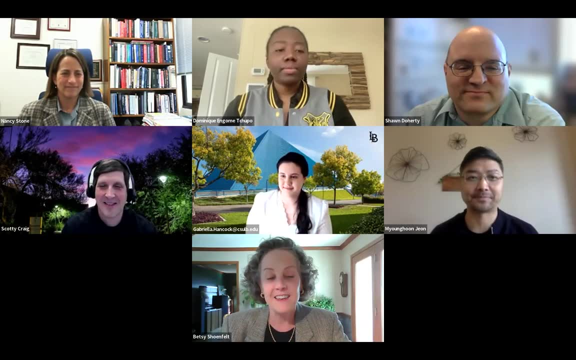 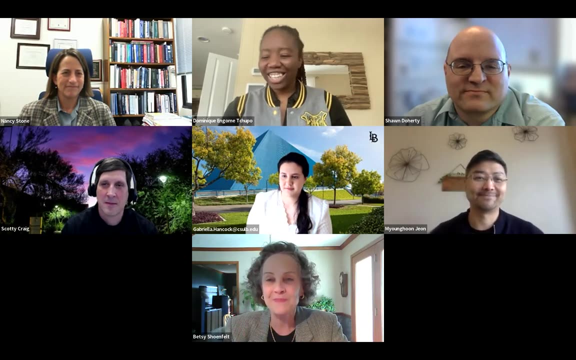 And so that's my one example of applied neuroscience, Thank you. Thank you, Gabby, That was really interesting. Next we have Dominique talking about team communication using cognitive fuzzy, cognitive mapping. Hi everyone, My name is Dominique. I am a fourth year doctoral student in the industrial systems engineering program, a PhD program at the University of Rhode Island. 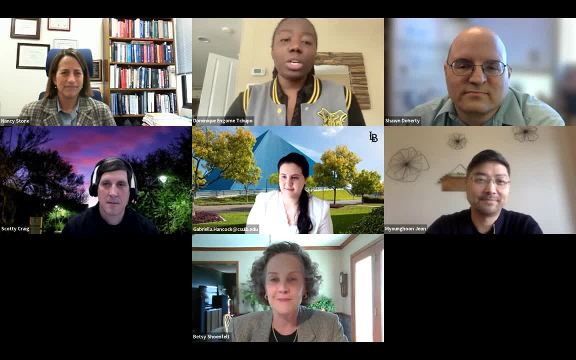 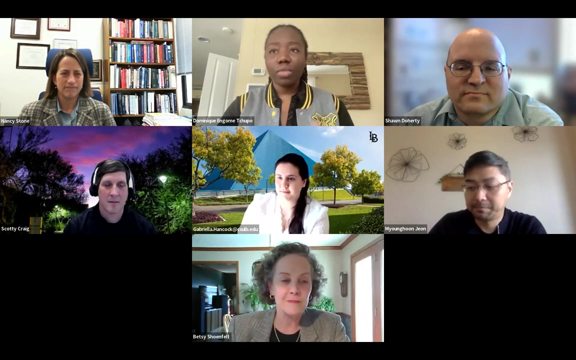 And, as Betsy said, I am going to be talking a bit about my research focuses, which is specifically team communication and understanding its relation to team performance. So, as many or all of us are aware, modern society work requires teams. Most of the things that are done today require teams. 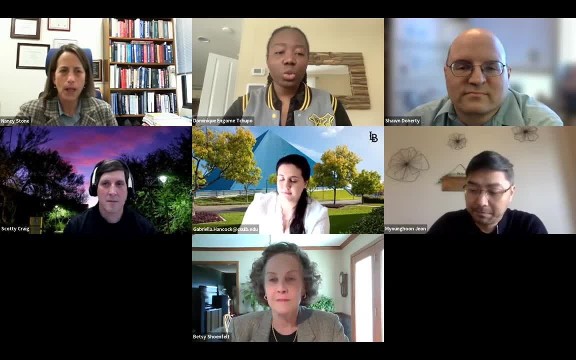 The tasks are just too complex to be performed individually and therefore require people of varied expertise to come together in order to solve different problems. If you look at surgical teams or construction teams, for example, these are not tasks that a single person can do on their own. 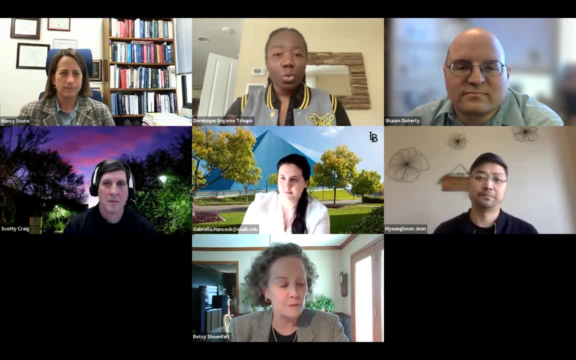 So you need a team for that And for teams to work together. they need to be able to communicate in some way, So they need to be able to share. They need to be able to share ideas, They need to make sure that everyone understands what the problem is and the various steps. 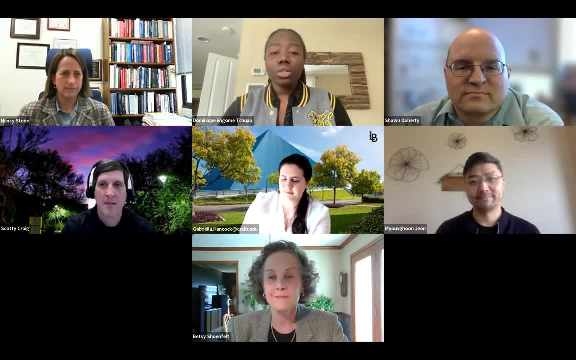 required to solve these problems And so to understand it. through much research and through just through observation, it comes to understanding that, in order to understand how a team works, we need to and how they attain the results they have. We need to understand how they interact or how they communicate. 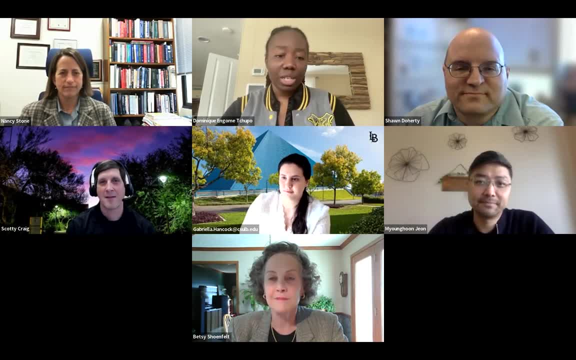 And so, for the past several decades, research has been done on understanding that relation between team communication and team performance, And some have attempted to do this using quantity of communication, to see if how much they communicate affects their performance, And that has, for the most part, been found to not be the case. 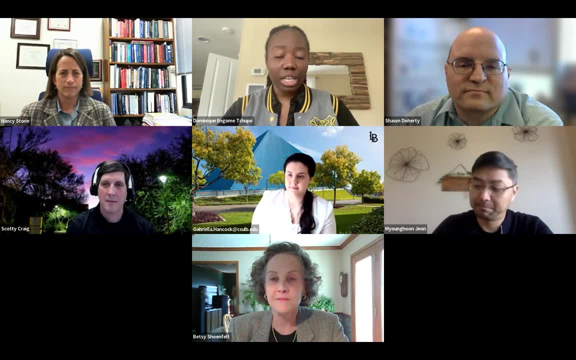 So my research proposes looking at the quality of the team communication, specifically the verbal aspects, so them talking, and trying to map the flow of the communication between the team members based on the type of message that's being sent. And by type of message here I mean whether they're asking a question, whether they're 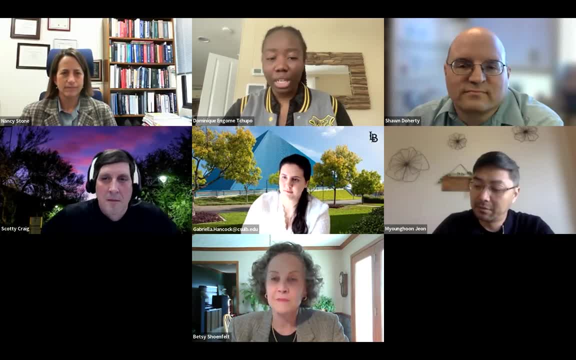 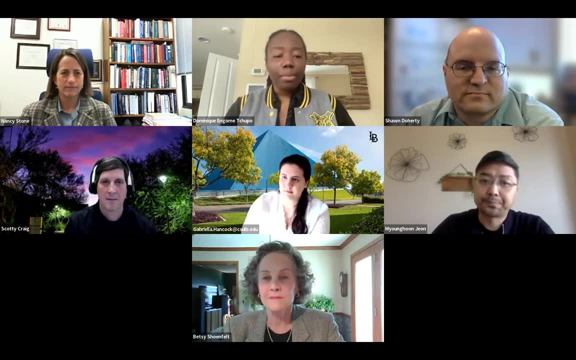 answering a question, whether they're just providing information unprompted or just making a random statement that has nothing to do with the task at hand. So those are the types of messages I'm looking at, And so, As was introduced earlier by Dr. 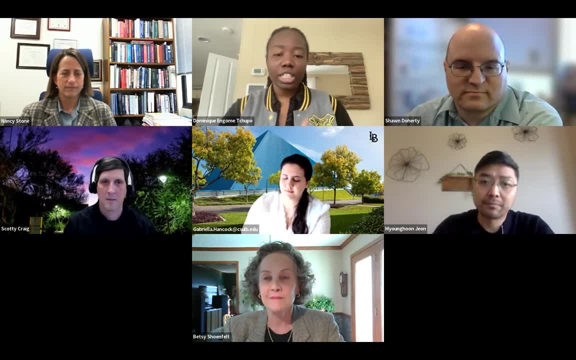 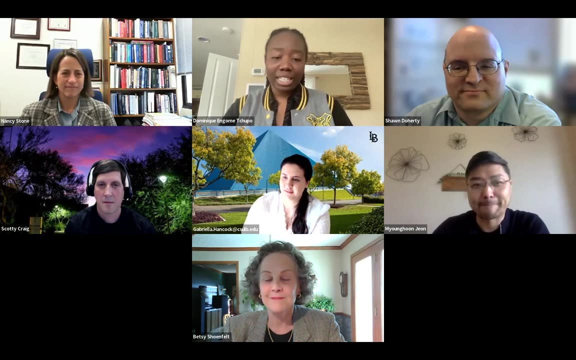 Stone, the field of human factor psychology is very broad. You can bring in a lot of different disciplines And, because I personally just love math, almost minored in math, but didn't. the method I'm using is called fuzzy cognitive mapping, which is based in mathematics and computer science. 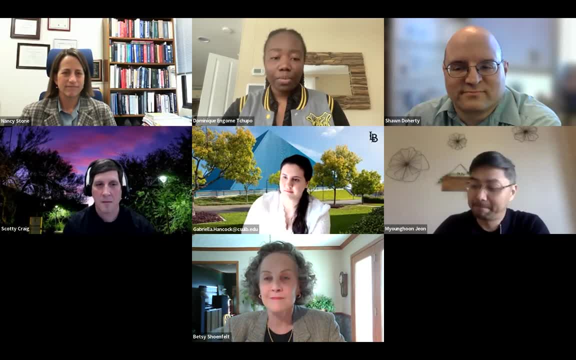 So I chose this method, because cognitive maps are already used to create mental models, So to create a map of what Of all, of how someone thinks through a problem. So, and essentially, team communication is a group's mental model. So it made sense to see if it could be applied from one individual but to not just for one. 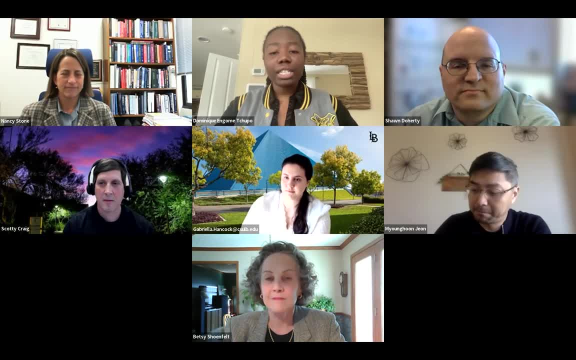 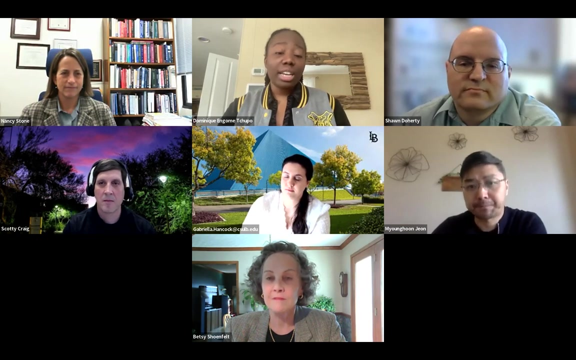 individual but for an entire group of people, And the fuzzy aspect in fuzzy cognitive mapping actually allows us to account for uncertainty. What this means is normally, when you have a Cognitive map, If, If you have concept a with an arrow leading to concept B, that means that a absolutely needs to be. no questions asked there. but we don't know that that is. that is always the case. 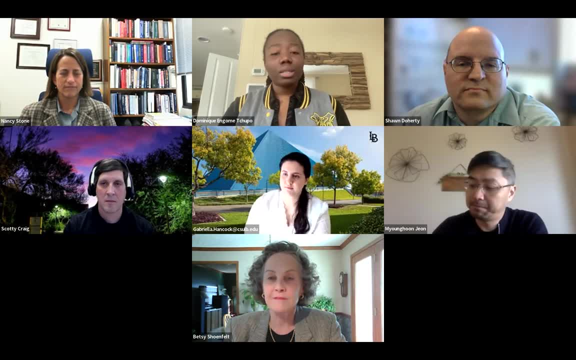 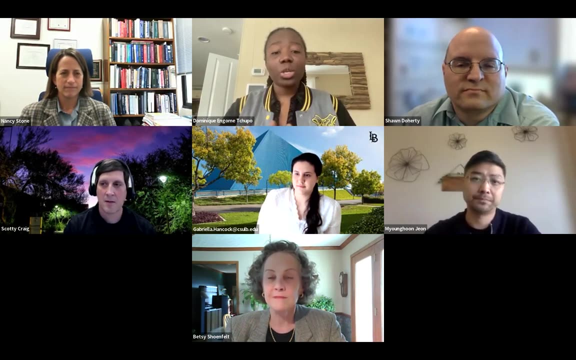 So The fuzzy aspect lets us be able to label this, to say that a might lead to be to some degree, and allows us to account for that margin of error and those unknowns. So my studies have been focused on demonstrating first Whether 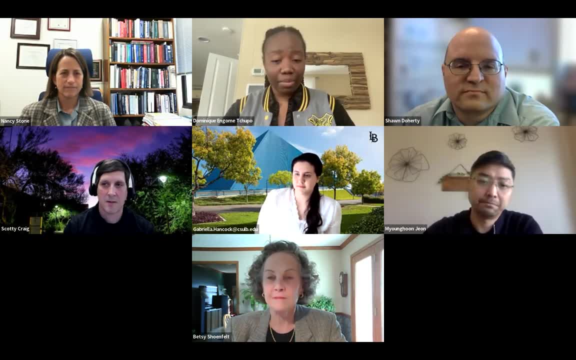 The method is viable because it's not actually something that has been attempted before, and how that works and just what kind of information it can tell us about team communication and how What patterns of communication lead to better team performances, because ideally we want all teams that are formed to do the work they need to do as well as possible. 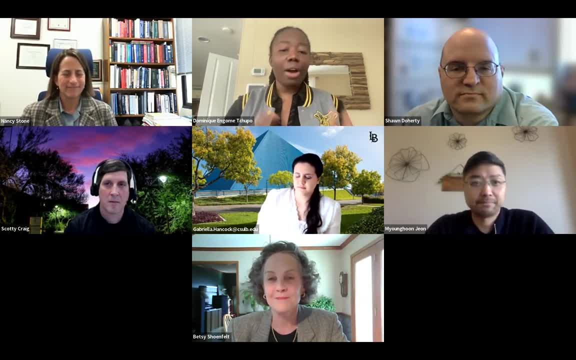 So Yeah, that's Kind of how some of my various Interest in mathematics led me to using those methods or methods in those fields to try and answer psychology questions, and hopefully that does give you an idea of how interdisciplinary not only the field is, but just one topic can be. 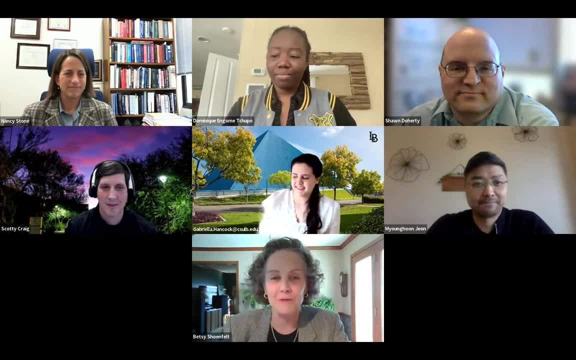 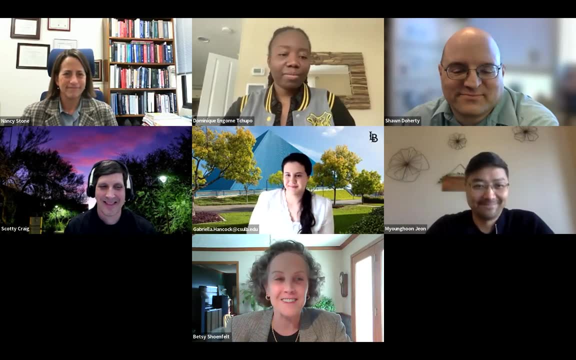 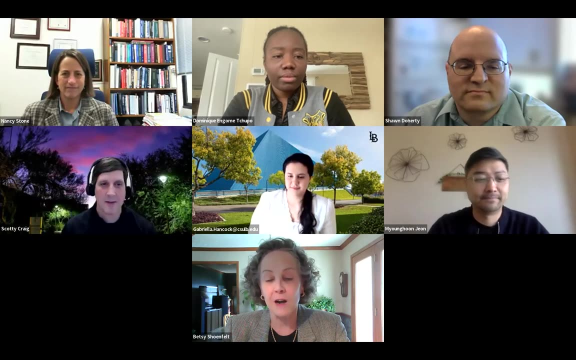 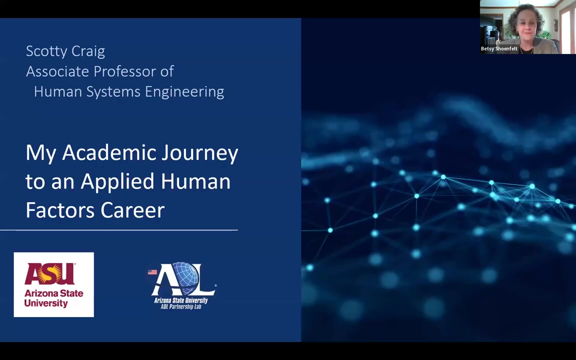 Thank you, You're muted, I know. Thank you, Dominique. That sounds like really important research. Good luck with it, Thank you. Thank you. Next we have Scotty talking about vicarious learning environments and intelligent tutoring systems. Hello, I'm Dr. 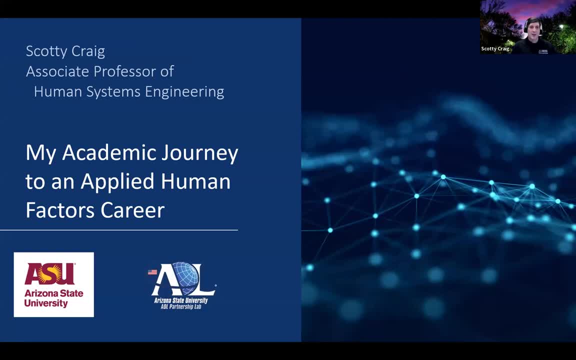 Scotty Craig. I'm an associate professor of human systems engineering at Arizona State University in human systems engineering area. It really is a human applied human factors area where we combine psychology, technology and engineering to help build systems that make humans more efficient. and today I'm going to quickly run through my academic journey to becoming an applied human factor or getting into an applied human factors career. 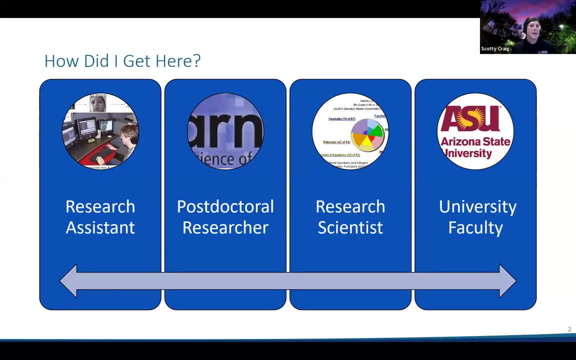 So how did I actually get here? So, starting out in the beginning, it may have been actually very questionable that I would actually end up As a university faculty member. I started out In a small town in the rural south in West Tennessee- about 2000 people. I didn't even hardly know anybody who went to college. I wasn't sure if I was going to go to college, but I wanted to explore it. 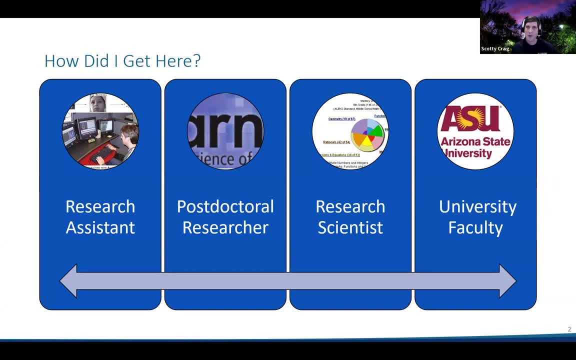 When I was in high school. so I actually reached out to a local university, the University of Memphis, and was able to get access to attending classrooms from that. I attended a class and got to meet Dr Wendy Rogers, who explained the field of human factors to me and cognitive psychology, and it ignited a spark in me. 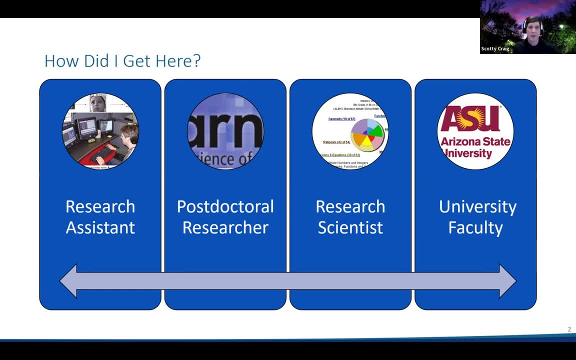 And so I did. I sort of. from that I went to college and I actually went into psychology and got a bachelor's in psychology, stayed on and got a PhD in experimental psychology, cognitive, focusing on education. During that time I actually got to work with Dr Art Gracer, who has been a wonderful mentor to me both as in the undergraduate and graduate, where I worked as a research assistant, and these are great positions where you get 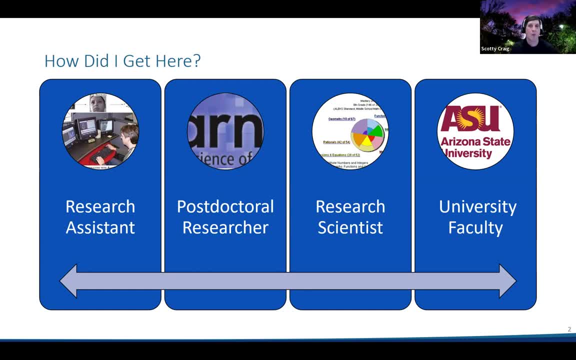 Even at the undergraduate level, you can work directly with faculty members and work on real research. What I got to do during that time as research assistant, both again undergraduate and graduate, is work on systems like auto tutor. Auto tutor is an intelligent tutoring system. 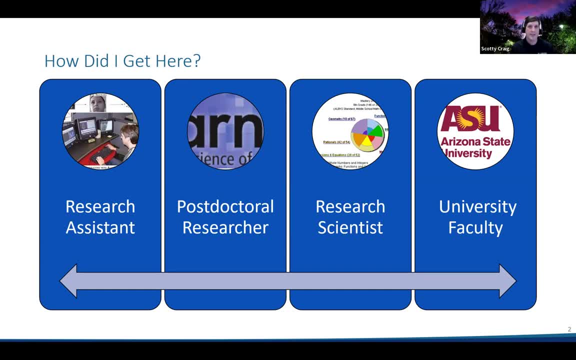 that tutors But like to the physics and computer computer literacy, it interacts in natural language with with the user to walk them through answering Problems- problems within the area. and when I was in graduate school we actually worked on. we expanded the auto tutor system to look at asset. 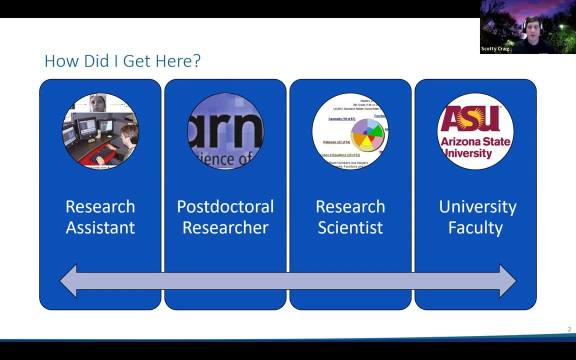 So the system cannot just look at how well they're doing as far the users doing, So the system cannot just look at how well they're doing as far as performance. we also used techniques such as facial expressions and body posture to detect emotions. the system could both. 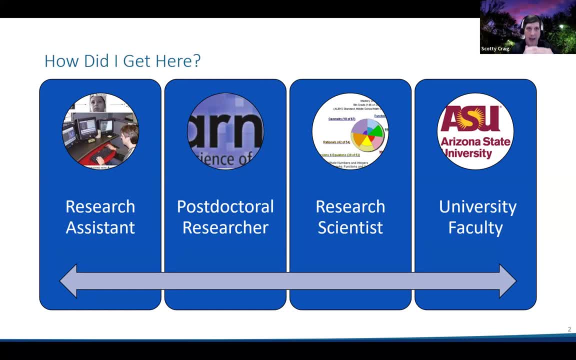 understand how well they're doing What they're experiencing emotionally and respond based off of that to improve and support learning. now, after that, after my PhD, I went on to another, which is very common- next level. I'm a training, which is a postdoc. 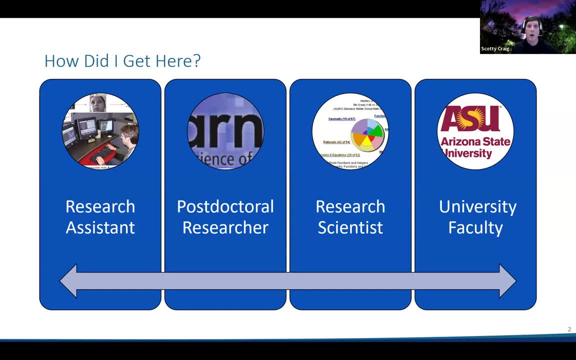 researcher but I worked for two years at the Pittsburgh science and learning Center where I learned- I learned- how to take what I learned about lab research and apply it in real world settings, specifically classrooms. So how do you conduct classroom research After that actually got hired back at the University of Memphis as a research scientist? now these are research focus positions where you really get to go out and get grants to do applied research and expand the field. 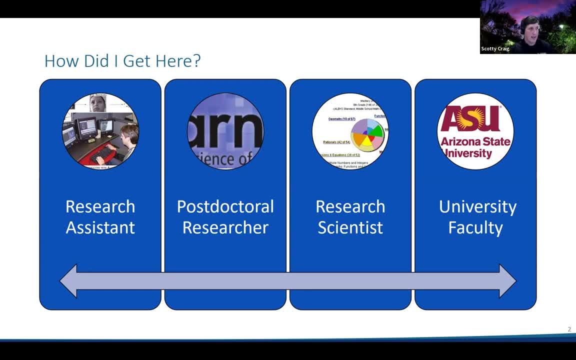 And in this area I got to go into, take what I've learned at the Pittsburgh science and learning Center and in my PhD Training and apply take technologies, specifically video based technologies, into classrooms. i'm to look at how we can design short videos, specifically focusing on the dialogue within those videos to prompt and reinforce learning and 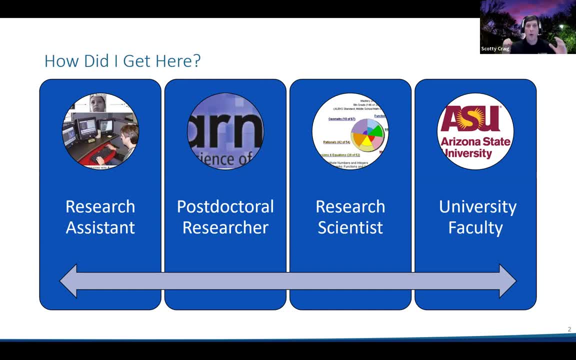 I got to work on another project During that time where I evaluated a piece of learning technology, the Alex system, within middle school mathematics after school program that was actually in Western to see school systems. So I got to go back to that same area that I grew up in and really give back with that training. after a few- about five- years of research scientists I moved on to. my current position is university faculty. 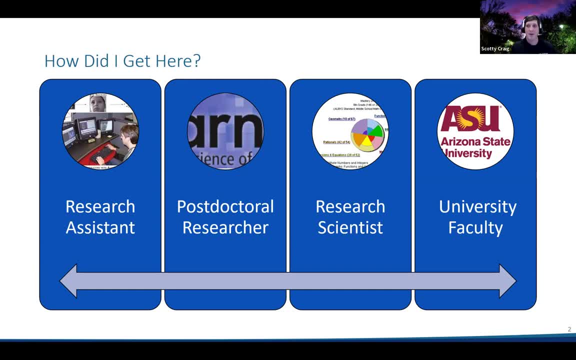 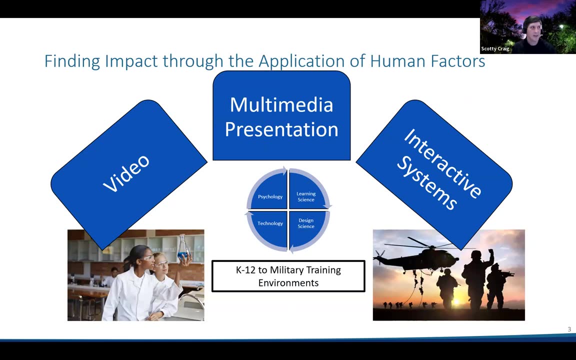 And you actually already had heard a wonderful example about that Earlier, about teaching, and when I get to teaching I get to do research and I get to do service to the Community to give back now from these fields. It was really exciting because what I got to do is actually find impact through the application of human factors in all of these areas. the way i've looked at it specifically, with giving feedback or giving impact, is through the implementation of videos. 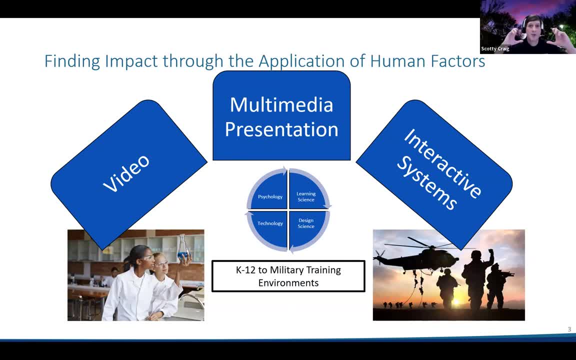 where we looked at how do you design these videos, specifically, structuring dialogue, using good questions and scaffolded questions to improve learning. interactive multimedia presentations: where you take might take these videos, but you also add in other types of feedback with them To to support learning and highly dynamic interactive systems, such as the auto to the system and talked about what people will interact in natural language. 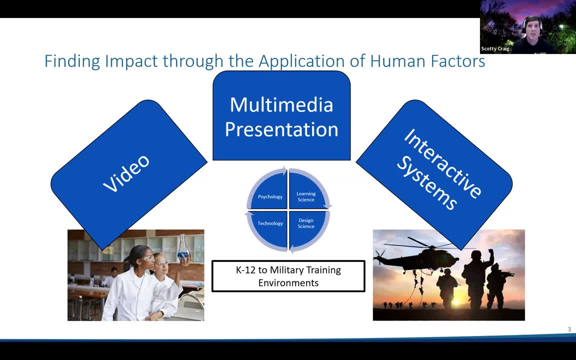 or other types of highly interactive environment. We bring in artificial intelligence to support learning, and i've been able to look at this From the K 12 level on to work that i'm working in now in the military area, where i'm evaluating learning technologies that soldiers are actually using in the field for their training. 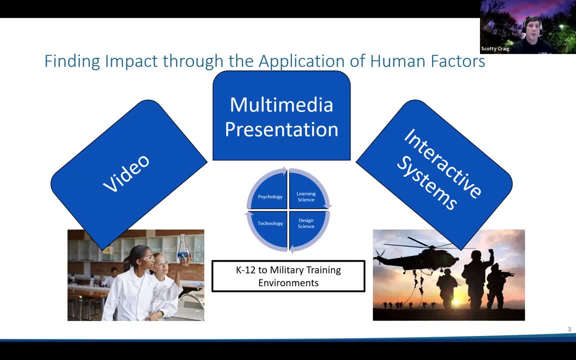 And, in closing, what this is allowed me to do within my career is to combine the areas of psychology, learning sciences, the design sciences, such as ux research and technology, to all within the area of human factors to have an apply and establish real world impact of applications. thank you, 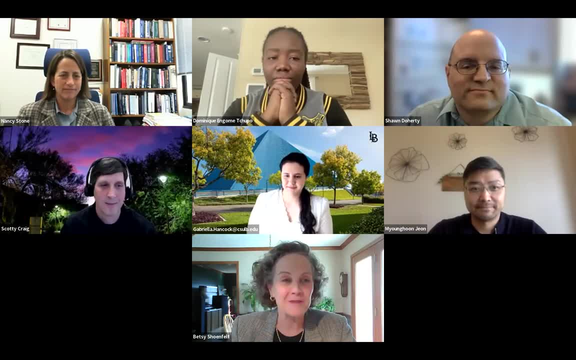 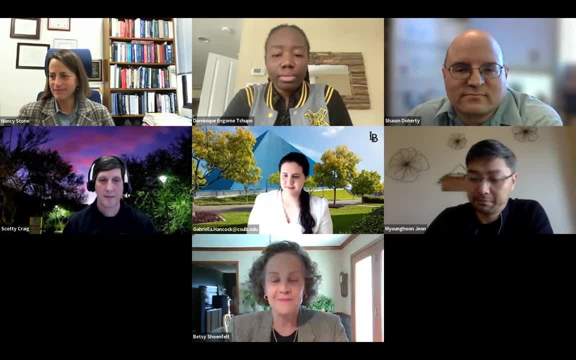 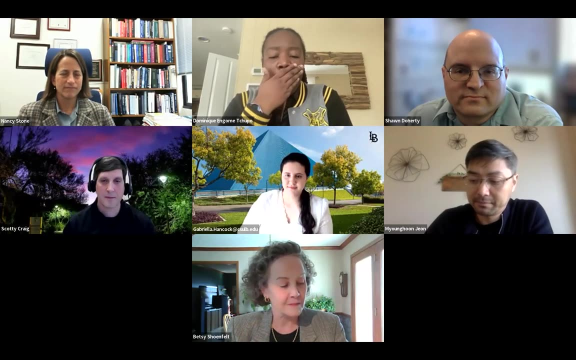 Now we have Rupa presenting on intervention supporting home health management. Thanks for the introduction and for organizing this wonderful panel, and so my name is Rupa Valdez. i'm an associate professor at the University of Virginia, with joint appointments In a few different spaces, so engineering systems and environment, public health sciences and global studies. 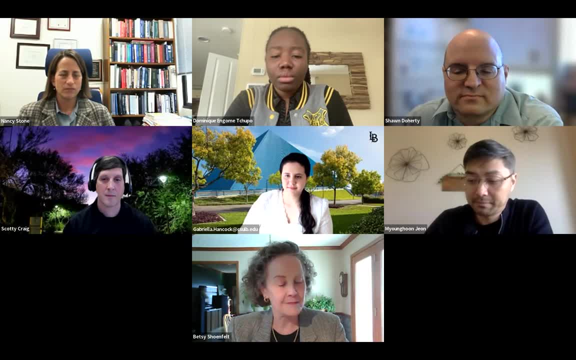 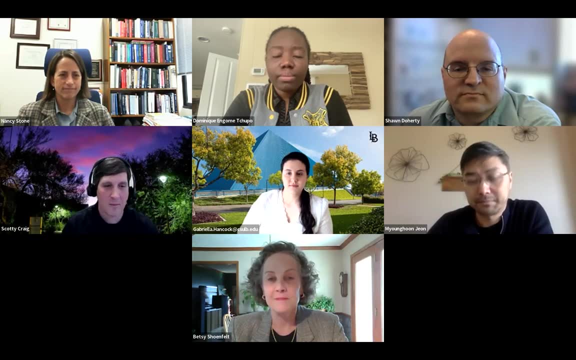 And, I think, my camera off. today i'll talk about this a little bit more, but I live with multiple disabilities, one of which is vision related with me, so difficult for me to look at screens for long periods of time. So you can think of this. 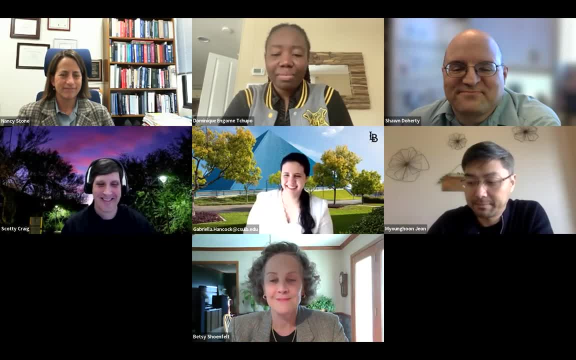 As more as a podcast for my part of the presentation. So I entered this space of human factors from an engineering perspective and, like gabby, I was originally influenced by my father, who is an engineer And, but, unlike gabby, who, you know, knew what you want to do and follow through with it. I thought I knew what I wanted to do and then realize along the way that I really didn't. 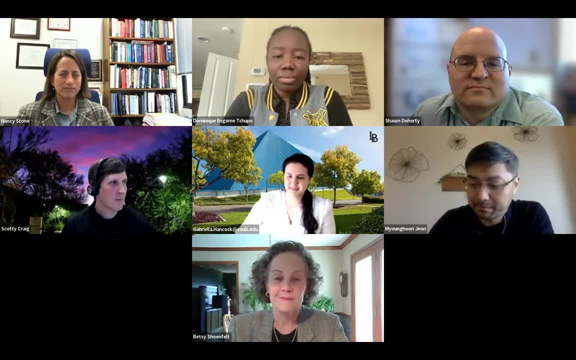 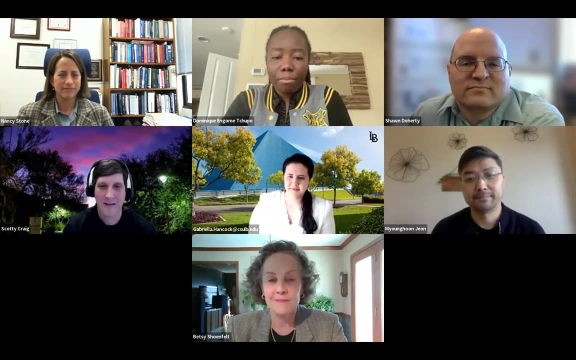 And so in my undergraduate degree I knew I wanted to go into engineering, And I don't think I was particularly sophisticated in my choosing of industrial engineering. but what drew me in was, in an introductory class, the idea that industrial engineering, and particularly human factors, synthesizes the technical aspects of engineering. 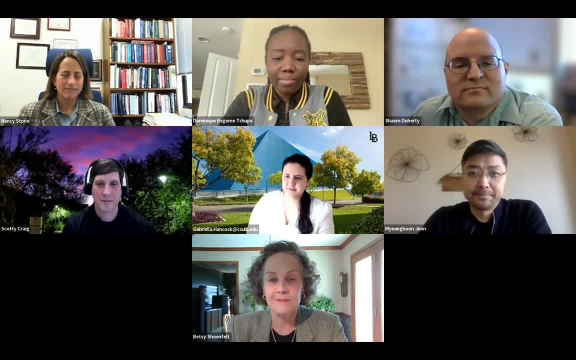 With skills and elements from social sciences and from business, and so I thought you know I would do this and I would end up working in consulting or working in some type of industry related position, Followed by doing something like an MBA or JD. 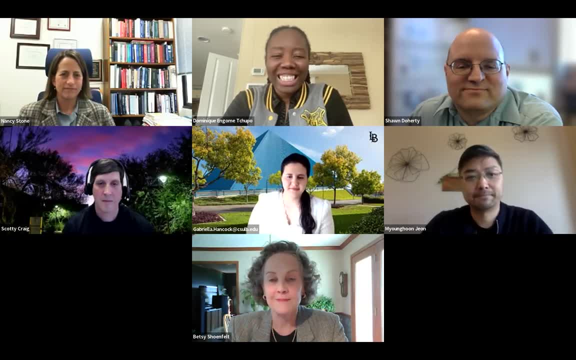 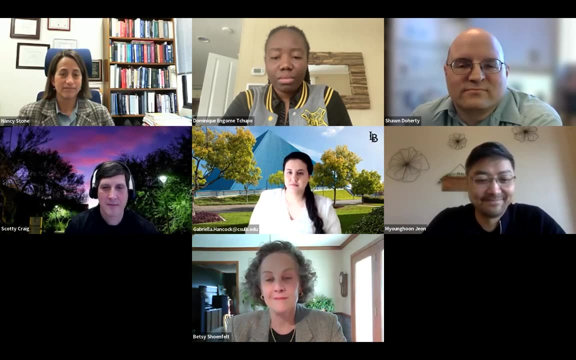 And I remember Saying quite distinctly that I would never go on to graduate school or do a PhD. so they'll never say never, right? So in sophomore year, though, of college, I acquired kind of the first set of chronic health conditions that I live with, and that was a, you know, quite a life changing experience for me in many ways, which sounds cliche, but, but yet was true. 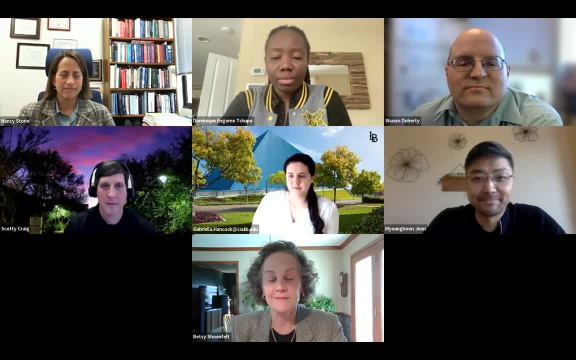 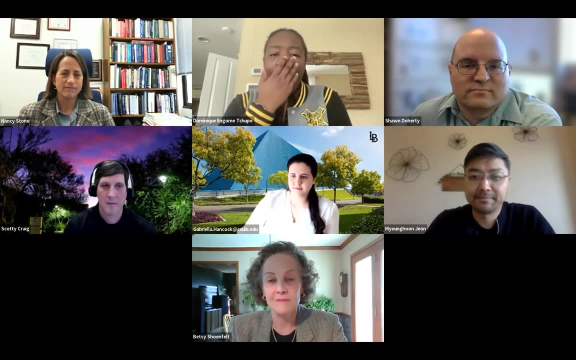 And I realized from my own experiences interacting with the healthcare system quite often, And after having not really had to do that for many years, that there was something there and that I wanted to Pursue. and I happen to be very lucky to be at Wisconsin at the time when there was a growing interest and expertise in human factors applied to healthcare. 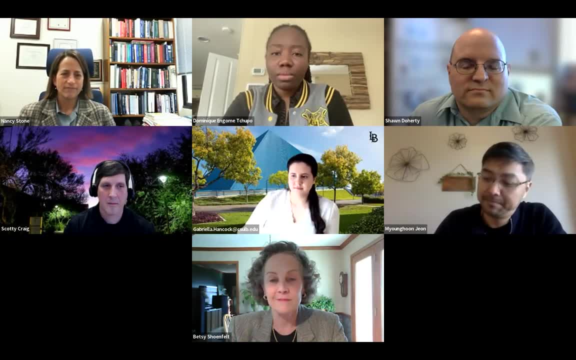 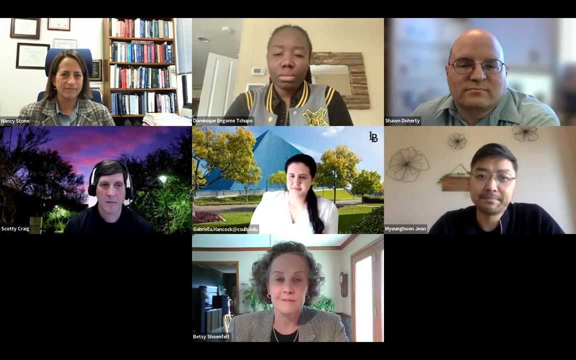 And so this was an opportunity for me to merge some of my personal experiences with a professional training I was just starting to receive. I went in and started doing internships in some pharmaceutical companies during undergrad, thinking that you know, it's still follow a path, kind of like I thought. but you know, in with a more of a focus on healthcare. 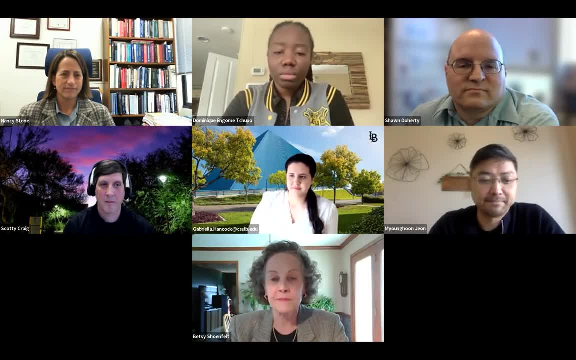 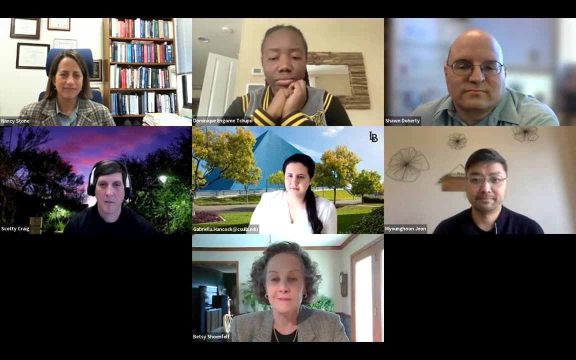 But after a few Those experiences and and feeling like that wasn't quite the right path for me and feeling there was some misalignment and values and priorities and kind of what I wanted to do and how I wanted to make an impact in healthcare, So I came into senior year feeling quite lost and in a serendipitous moment so sitting outside a professor's office waiting for him to begin office hours and heard him talking about some research in a home and community based space, working with women who are colorblind, and I remember thinking that's the kind of work I wanted to do. 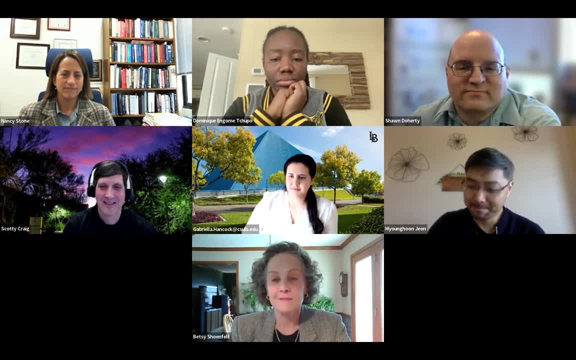 And so it was the first conversation I had about what would it mean to go to graduate school. that's not why it showed up to office hours, but that's what the conversation ended up being. So after undergrad, I took a few years and worked as a research intern, just trying to figure out if this was the path I wanted to follow, and realize that it was. 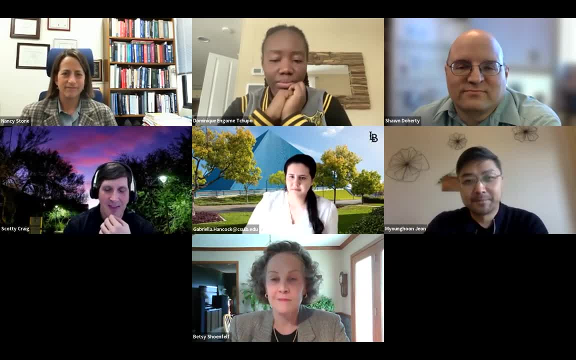 So in graduate school I pursued also a degree in industrial and systems engineering, so kept the engineering framing of this work in human factors. but the other thing i'd like to add in is both an undergrad and graduate School and talk about wandering off engineering campus quite a bit. so i'm particularly kind of majoring in multiple things in undergrad that were humanities related and then grad school spending a lot of time in a cultural anthropology department. 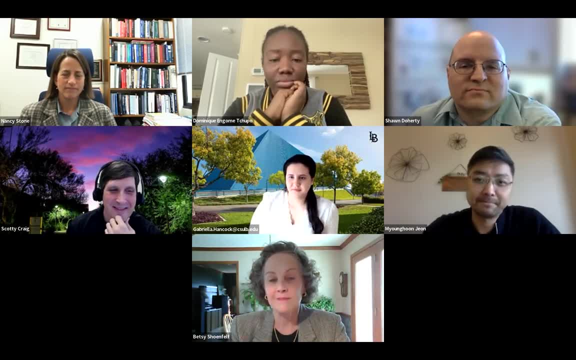 Because we talked a lot about user centered design, but I felt like I really didn't know how to interact in community and home spaces, which is what I wanted to be doing. this is a place I could go to learn about it, So now, as a professor, my work is really integrated across many disciplines. I talked about engineering and human factors. 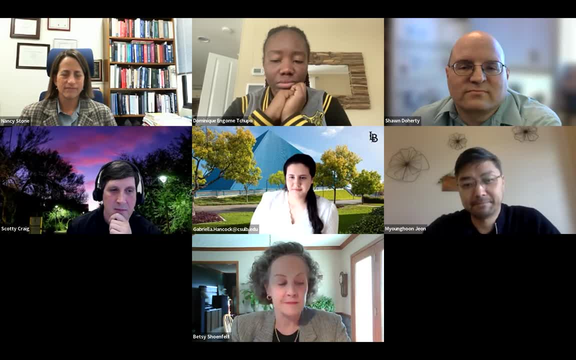 Health sciences and cultural anthropology. I do informatics based work so I like m health applications to support people in the home and community. A lot of this- disability studies, Community engagement- so sometimes he's like alphabet soup of disciplines, but part of what I love about human factors. for me it was a 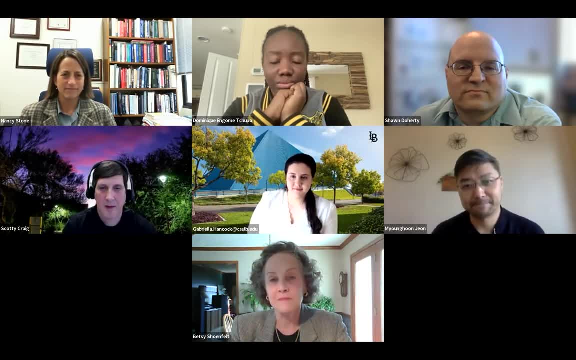 entry point into doing this multi disciplinary work and i've been able to explore other interests and learn from other fields along the way And, if i'm kind of, human factors- a space for professionally in terms of the discipline, but Also in terms of a Community that's really open to thinking about new techniques and how we might integrate across disciplines. 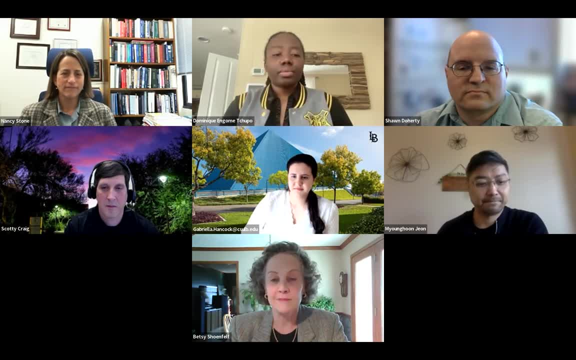 So my work focuses particularly on how chronic health conditions are managed and home and Community based spaces And everything from original we call needs assessment and the design process, so really spending time in people's homes and communities and learning about What those processes look like to design. a lot of my work is very Community engaged, so I work with the people i'm designing for to create solutions, whether those are technology based. 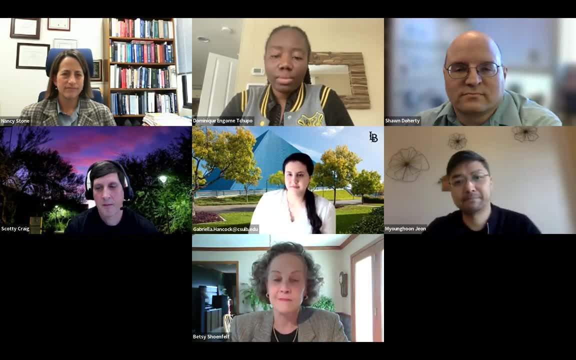 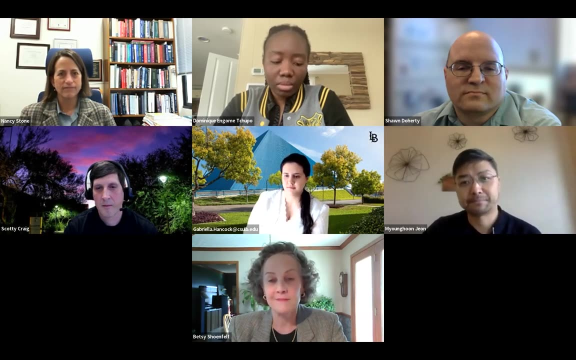 Or kind of broader systems, and then through evaluation Again, which is often a very participatory process. Most, almost all of my work is focused on groups that are under represented or left out of our traditional design efforts. so we talked about this in healthcare is health disparity populations. 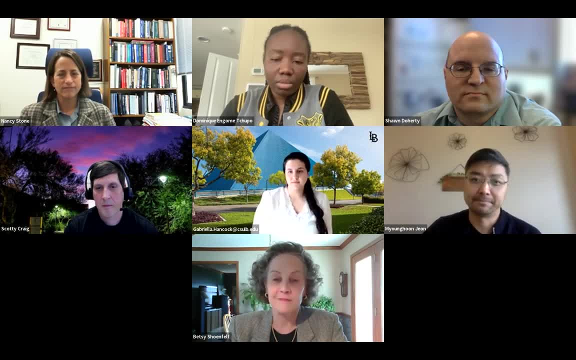 So originally focused predominantly on thinking about racial and ethnic minorities, and that work has moved into a lot of different health disparity places. so, For example, I do a fair amount of work with The Disability Community. I do a lot of work again with our public housing Community, with 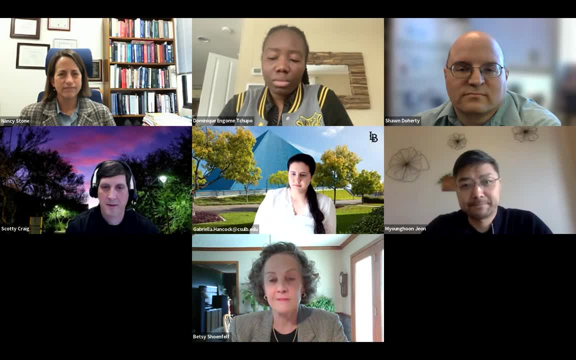 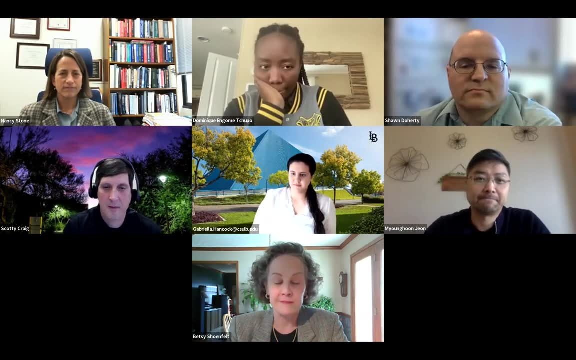 Communities in South Africa and India that are also under resourced, And so my research isn't in this space, my teaching is also, and what I love about the teaching I get to do is that it's also tends to be very interdisciplinary. having students from 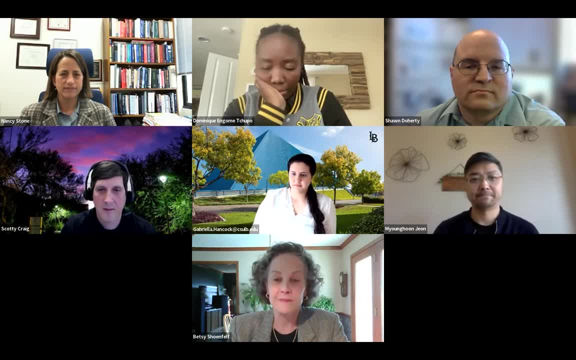 Engineering, from public health, from social sciences, come together one classroom, and so it's not that they're just learning from me, they're really learning from one another. And then the last part i'd like To say is that another kind of wonderful thing that I think a human factors allows us to do is we often talk about creating alignment right, and we've heard about creating alignment dimension. the person that are physical or cognitive in nature. 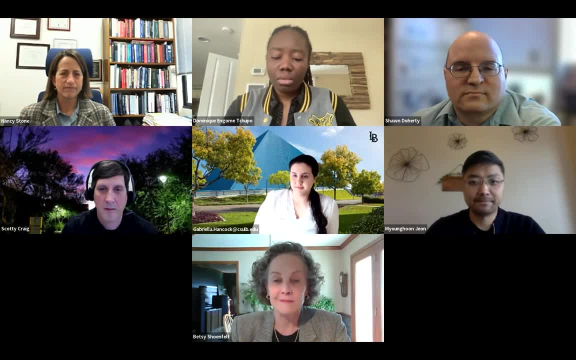 But as someone in the sub discipline called macro ergonomics, I think a lot about putting alignment between the person and the broader context that they're embedded in, so Now that their immediate kind of physical environment, but also looking at their social environment of their family or their community, looking at their cultural 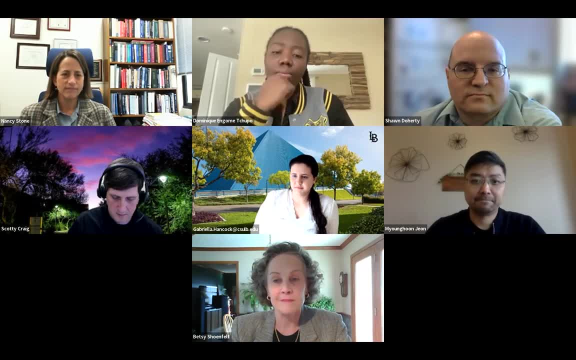 Beliefs And then kind of broader Policies in place. and so, as i've kind of grown in my career, focus not just on the creating alignment But also thinking a lot about how we might change that broader context, especially when we're looking at questions of health, equity and social justice. 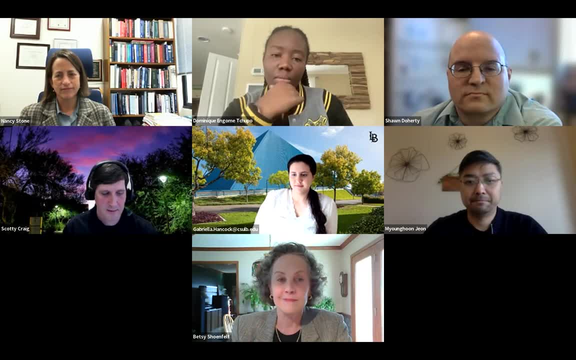 And so that's to say that my career has also increasingly included a large advocacy component as a part of the work. I do so with that. that's the. i'll turn it back over to you and I hope for all the students this is continue to build your interest in exploring human factors and the many ways that it can be applied. 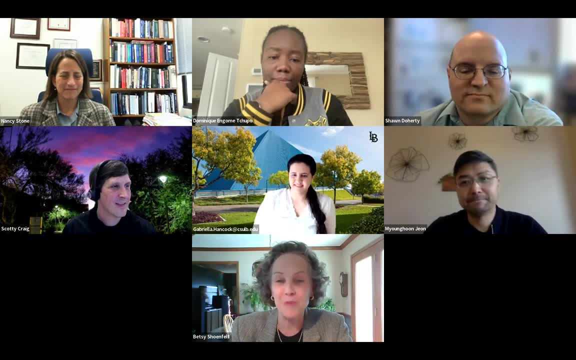 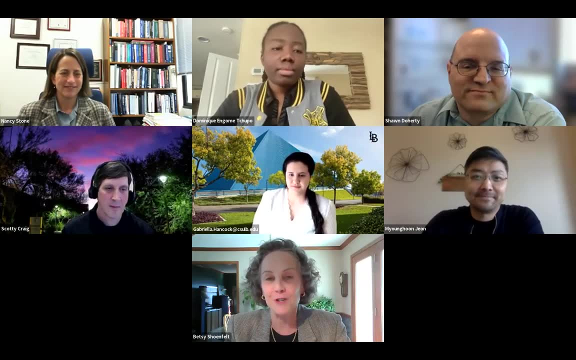 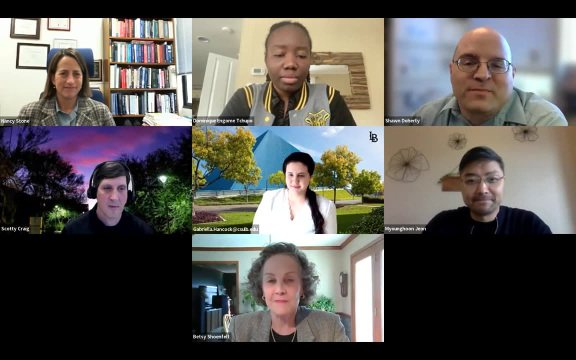 Thank you, rupa. some really, again, interesting and important work. thank you so much. Now Sean will speak on gaining gamification and virtual reality. hi everyone, my name is Sean doherty and i'm an associate professor here at Embry-Riddle Aeronautical University. 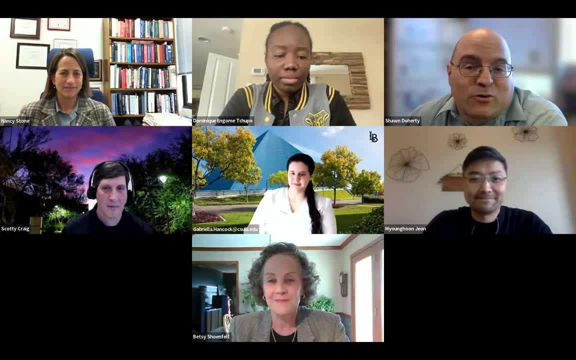 And if you're watching this video, then you already have a leg up over many people that are interested in human factors, because most people don't know the term human factors, And I certainly didn't when I started out in my educational path. But in high school I did know that I really liked psychology and I really liked computers. so when I went off to undergrad 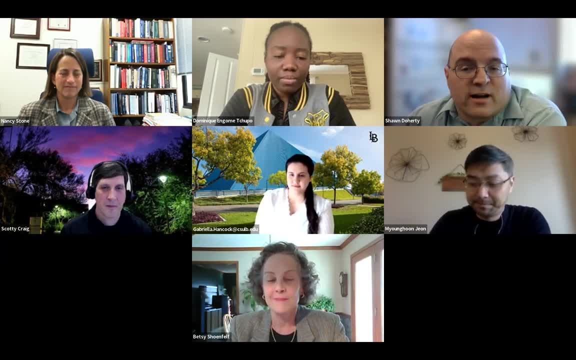 To get my undergraduate degree I did a double major, both in psychology and computer science, and at the end of that I realized I kind of like academics. I wanted to go on for some more graduate work, so I went off for my master's and my PhD at an institution that had human factors research. 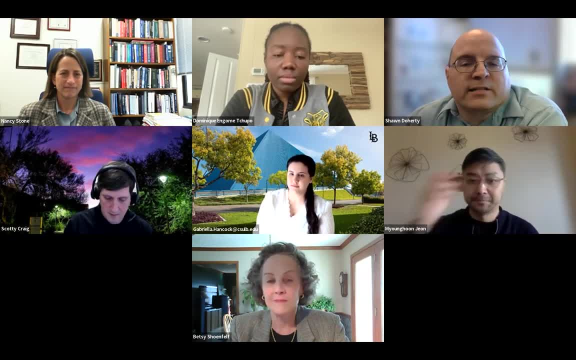 largely in aviation. they did a lot of work looking at design and application of the interactions between pilots and the equipment of pilots within the aviation industry, And so after that, by that point, i'd fallen in love with academics and I sent around a bunch of job applications and I got a job offer here at Embry-Riddle, where i've been ever since and love it. 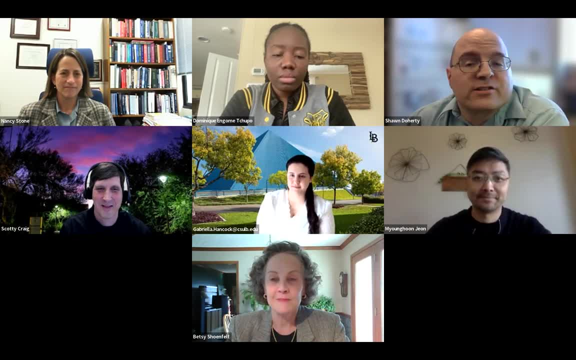 And it was largely because I had that background in human factors and psychology and aviation at an aeronautical school That got me in the door, and so I spent the first portion of my time here at Embry-Riddle doing typical faculty things and researching aviation, and there was a point in time. well, basically let me state it this way: 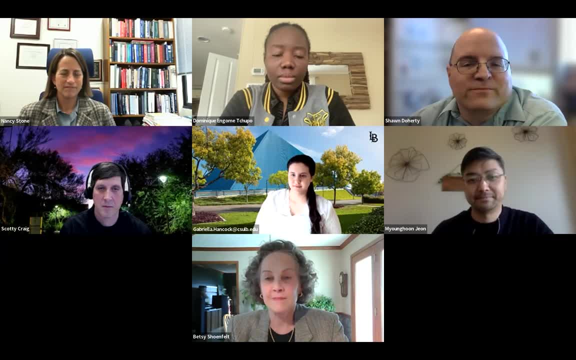 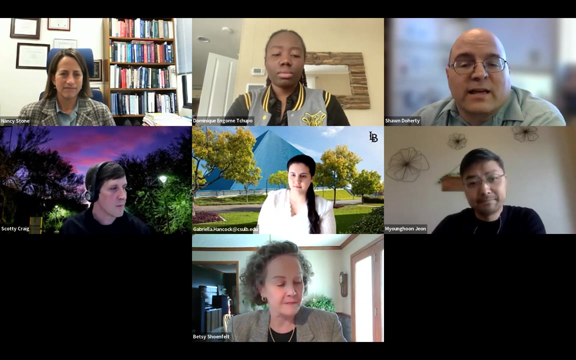 you've heard a little bit from some of the other faculty on the call here today of kind of what our average day is. It involves three primary things, where one of them is teaching, and I teach primarily human factors classes, Either on basic processes related to perception or attention or cognition and so forth, but also different kinds of techniques or domains such as the domains of aviation or air traffic control or entertainment systems, and looking also at other domains such as medical or 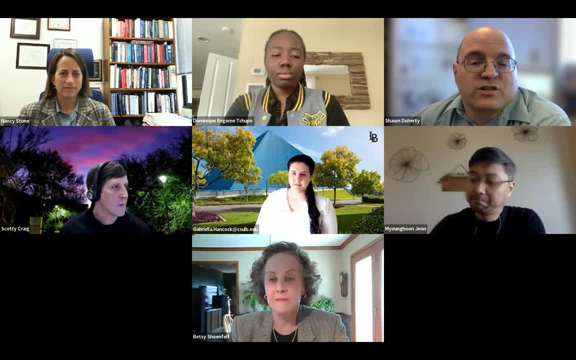 things like safety or automation and so forth. so teaching is one part of it. Service is another Where, in my case, I spent a lot of time- as I suspect many people here on the call do- in terms of meetings and helping out our colleagues and students and so forth. 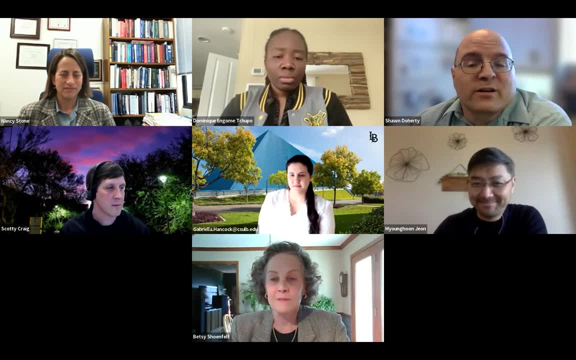 In terms of assistance at the department level or at our university or at the national level, already related to human factors, and, in my case, one of the ones that is specific to my service component is that I am our internship advisor here at Embry-Riddle. 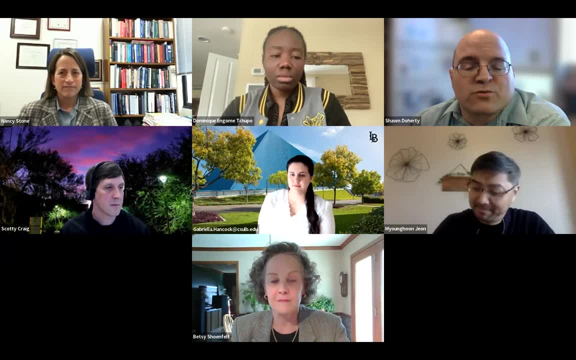 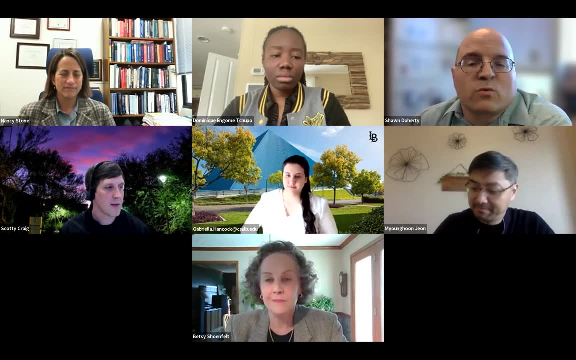 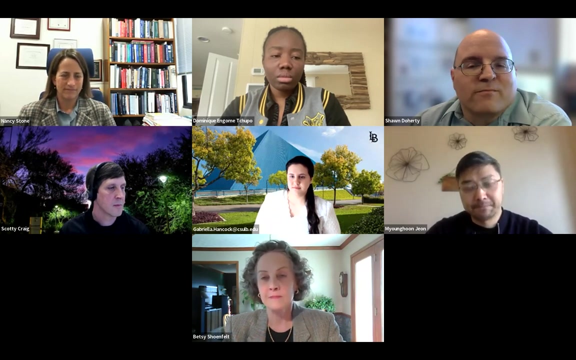 And so I oversee our students that go off and get internships where they go off to a company and they gain experience with human factors while they're completing their Undergraduate work, which hopefully, or graduate work that will hopefully transition to a career in human factors, and so they go off and do internships related to transfer, transportation, such as aviation or automotive. they may go out and work in. 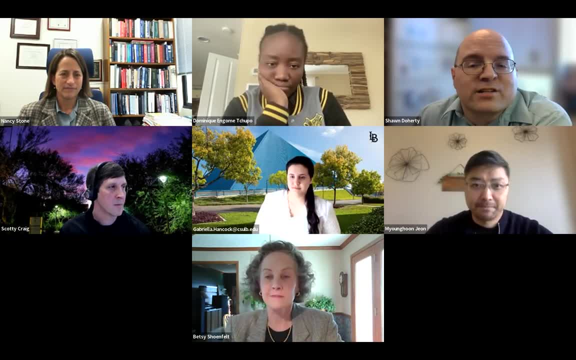 In manufacturing locations, locations. They may go off into medical areas, They may do an internship with government, They might do an internship with some research companies. It's a very broad set of directions that our students go, just as Dr Stone referred to at the very beginning in terms of just the 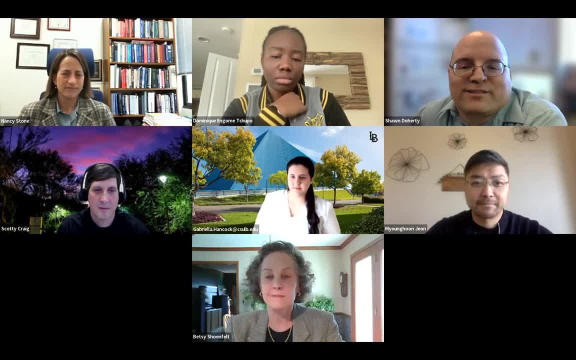 broadness of our discipline And I get to see all of our students go out and, you know, have these wonderful experiences with these companies that hopefully transition to careers. And then my third area is, like everybody else has talked about, is in research And I mentioned that I spent the 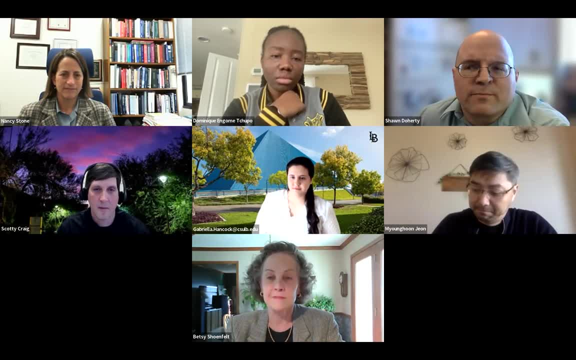 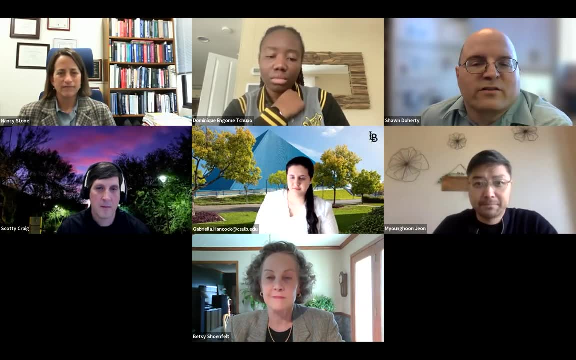 first portion of my career in aviation research And there was a point a number of years ago where myself and some of our colleagues were sitting around the department and talking and we all kind of looked at one another and realized that we kind of wanted to take our research in a 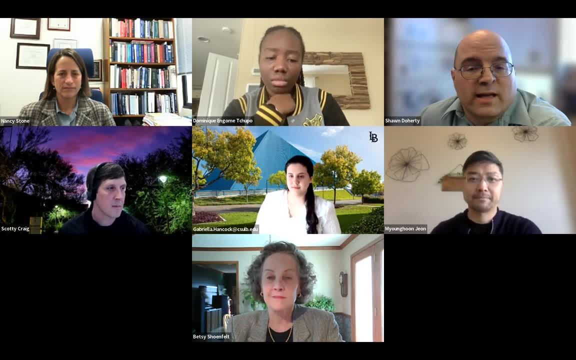 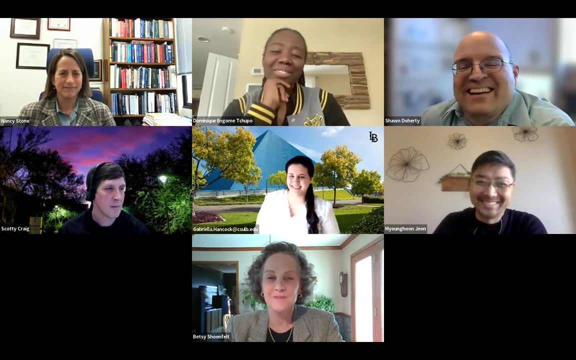 different direction And in talking a little bit more, we discovered that we all had an interest in games. Myself, I am a video game player for decades now And so very interested in video games and that interaction between the players and the. 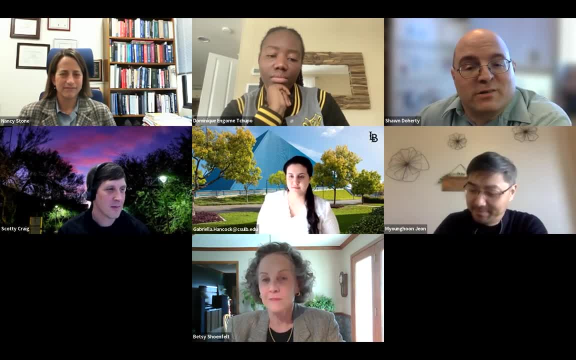 technology, So as with human factors, is that interface between people and technology? In my case, that technology is entertainment systems, And so my colleagues and myself use video games or other entertainment systems to look at basic behavior in people as they use those systems. or 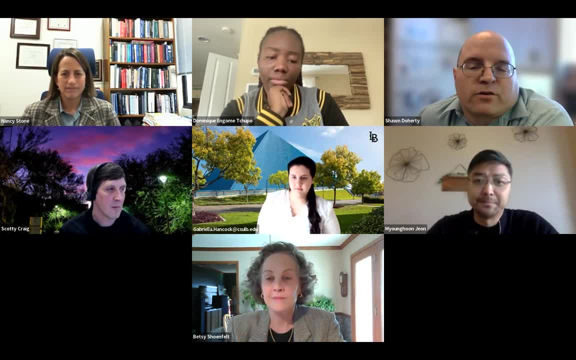 look at just the actual gameplay itself. So, for example, if you're a video game player, you're going to want to look at social interactions between people. That is, how do you build friendships? What kind of friendships do you have? Are they the same or different? online versus. 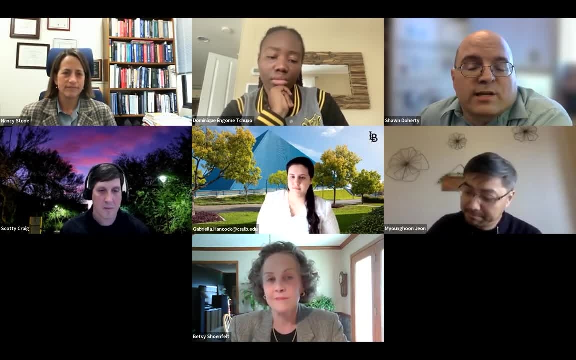 offline. I have another colleague that looks at video games and your experience with them. That is when you first get a video game. what is it like when you first start engaging with it? Do you like it? Are there things that you don't like? Would you be willing to buy another game like? 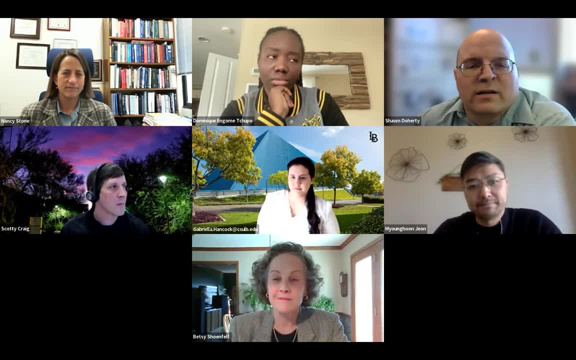 this And so, for example, I recently bought a video game. I bought a video game. I bought a video game. I recently played a game where the human factors design on it, I'm afraid, wasn't very good, where I started the game and all of the text in the game was dark, red text on a black. 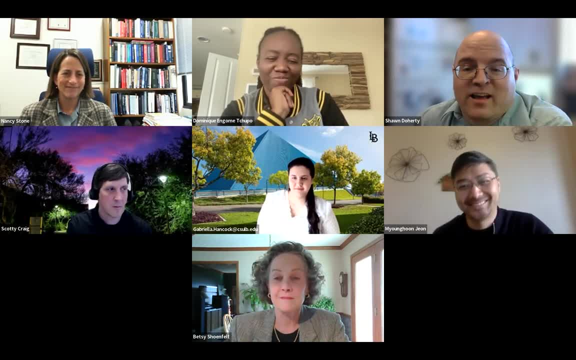 background in really tiny font. I love video games but I just could not play it. Not very good human factors design, And so my colleague works with some of those issues to try and improve overall game design. I have another set of colleagues that look at teamwork. 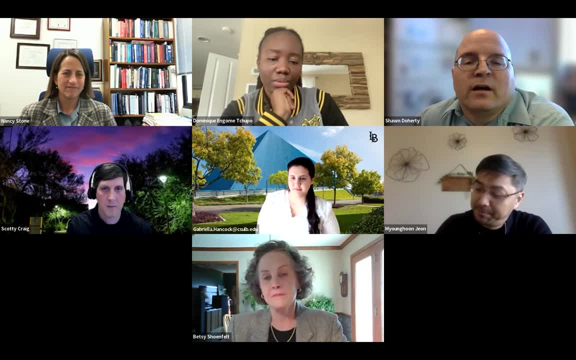 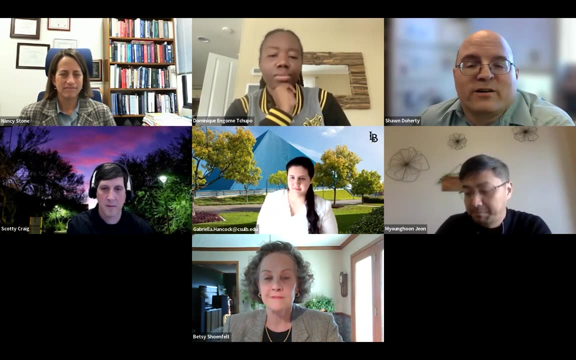 By using video games to try and understand how people work together, utilizing games as their platform. And myself personally, my area of research- I'm interested specifically in entertainment systems. That is, what do people enjoy? Why do they enjoy it? And so pretty much. 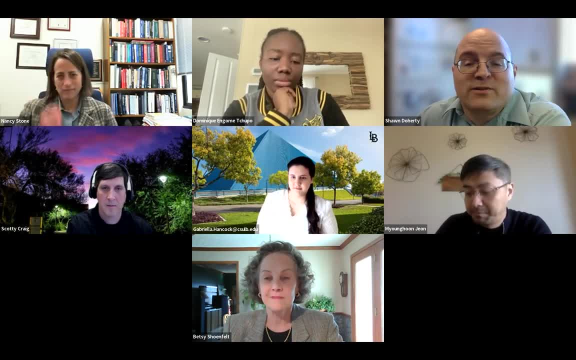 anything related to people interacting with some sort of entertainment system. I'm all over that, And so I research things like escape rooms, which is where you put a bunch of people in a room and you lock it and give them a whole bunch of puzzles and tell them that they can't get out. 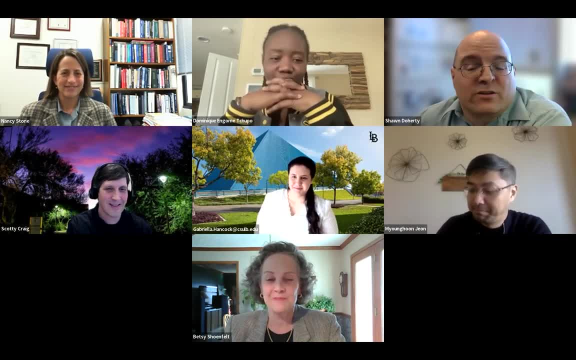 until they've solved all the puzzles. And so we look at, we use that to look at teamwork. I also look at things like expertise in video games. What makes one video game player much better than another, For example? I've been playing video games for years, but I would not. 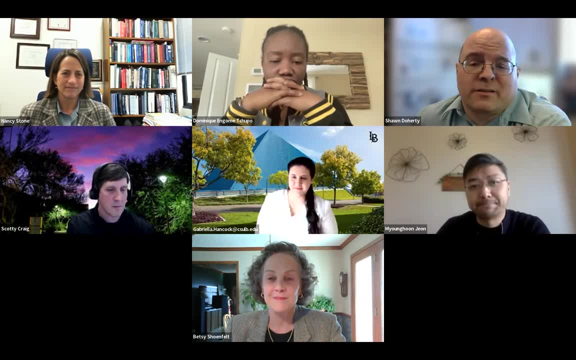 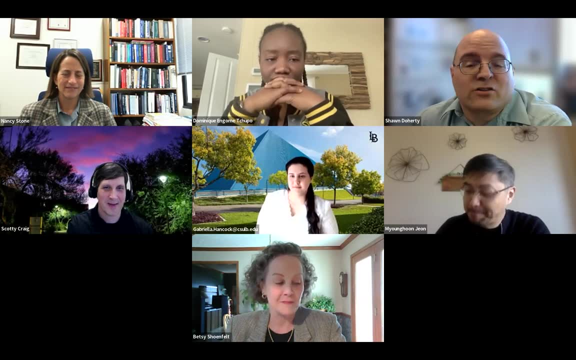 be useful on your first person shooter team. I'm nothing more than cannon fodder. I'm not very good, But so what does make those people that are very good at it? I also look at cheating behavior in games. What are the motivations for people? Why do they cheat? 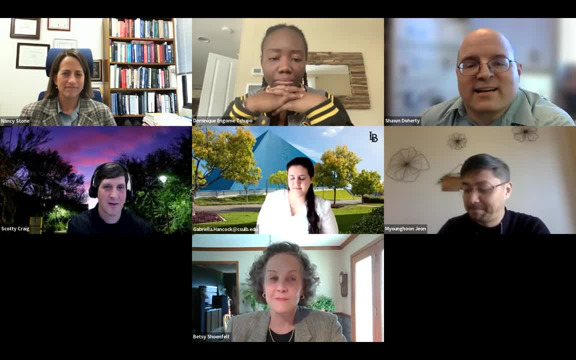 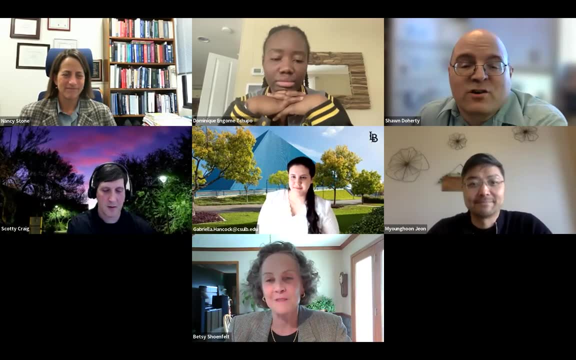 What gives them that opportunity? Do they take that opportunity? I look at some of that, And so I also do some research on gamification, which is taking the things that make something a game and applying it to things that aren't a game to try and make them more game-like. 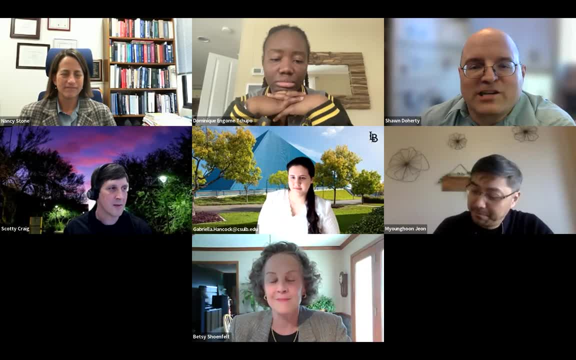 So if you've ever tried to play a game where you turn, you're studying into a game in order to make it a little bit better, well, that's gamification. And the last one is: I'm really interested in virtual reality and some of the effects that 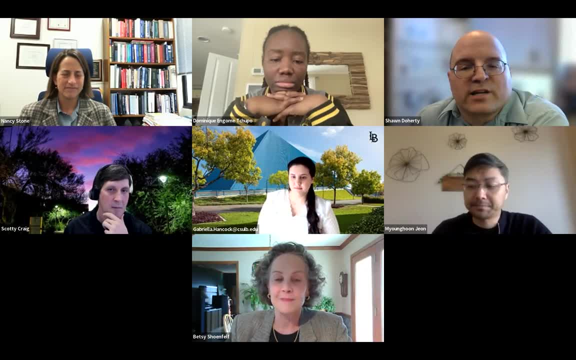 virtual reality has. So, for example, there's some evidence that suggests that we have some distortions in time and our perceptions of time when you're in virtual reality, And so those are the kinds of things that I do for research, which, personally, I enjoy a lot. 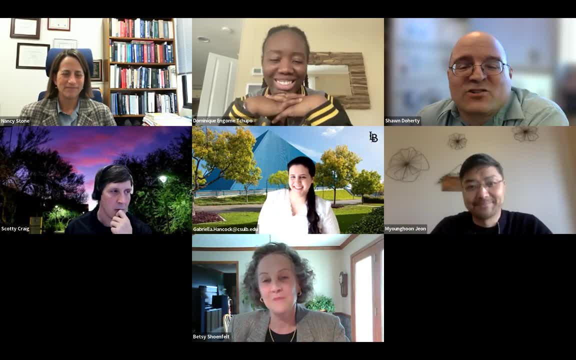 and I think are awesome and I've got a great job. And so if you're interested in this interaction between people and equipment, whether that's medical or in home design or educational systems and the other things that you've been hearing here, if you like design, if you like people, 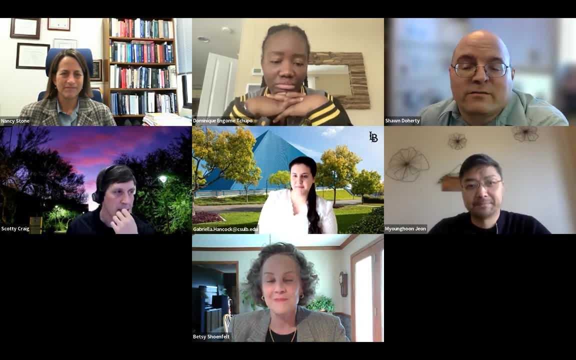 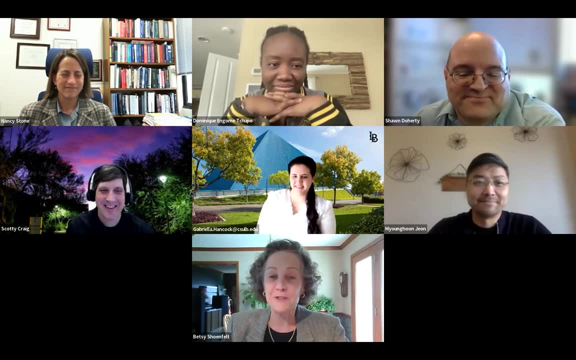 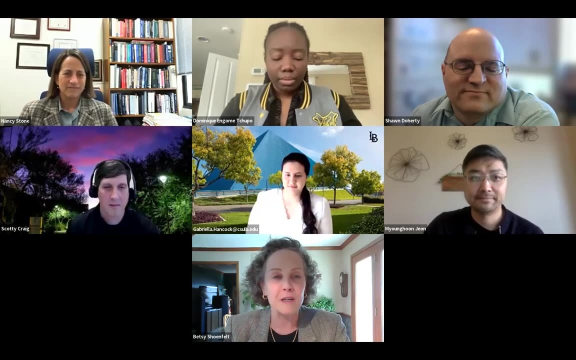 if you like technology, then maybe Human Factors is the right career for you. So thank you very much. I'll release the floor. Thank you, Sean. That sounds interesting, but also like a lot of fun. Now I'm going to ask each panelist for a final comment perhaps, which? 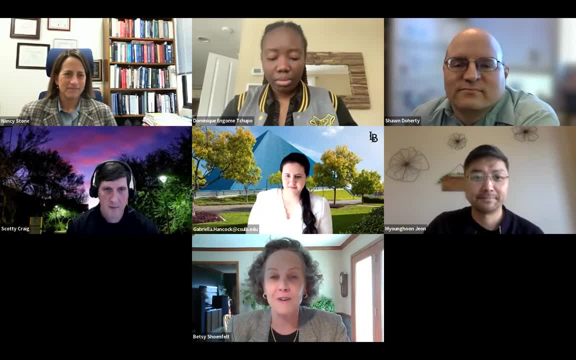 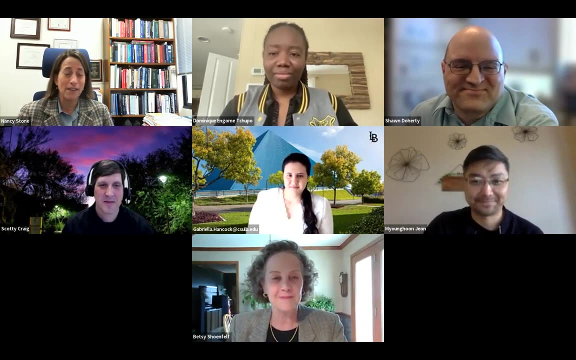 what they wish they knew before they started graduate school, or some other helpful insight. Nancy, All I could say is I really wish this video existed when I was looking for schools, So this has been really, really informative for me, So I think this was great, Great to. 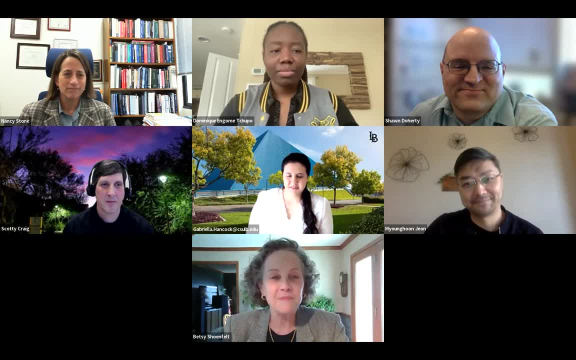 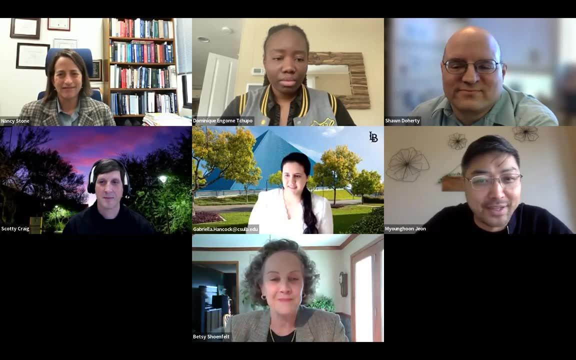 learn about my colleagues and their paths that they've taken. Yeah, I have one quote from Dante. It says: if you want to learn more about your path and let the others talk. So there are a bunch of different opportunities you can pave the way for yourself. 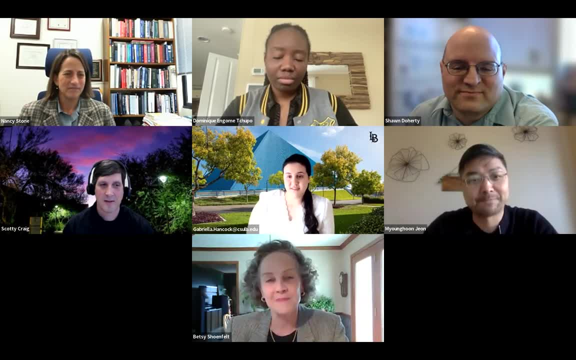 Gabby, The sky is really the limit with Human Factors, and grad school is what you make it. Everyone will have taken the same classes as you. It is your research and the other skills that you develop that while you're there that's really going to make you unique and set you up for a successful 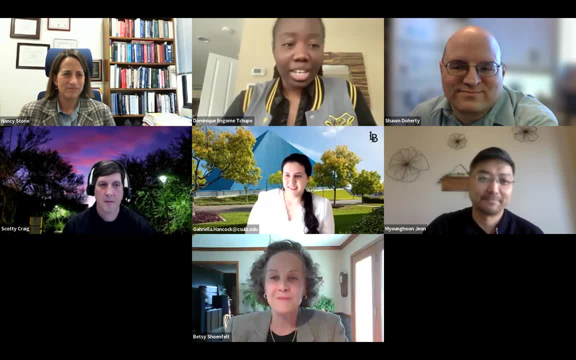 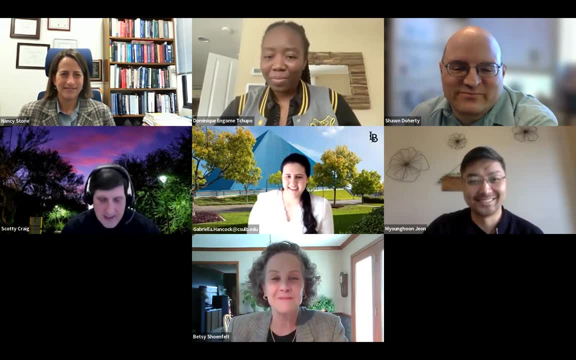 career, Dominique, And I forgot it immediately. Okay, let me circle back to you then, okay. Okay, Scotty, Yes, hopefully, what you kind of got from my talk is that it's really important to kind of foster your networks. You're not doing this alone within Human Factors. We work as groups. 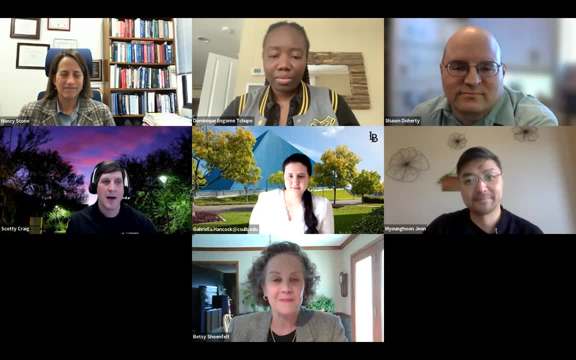 we work as teams, Find your mentors and find your colleagues, And they will be the support group that will help you form a much more successful and enjoyable path within this area. And the other thing to remember is that, hopefully, that you've seen is that Human Factors is flexible. You learn a lot of core basic skills. 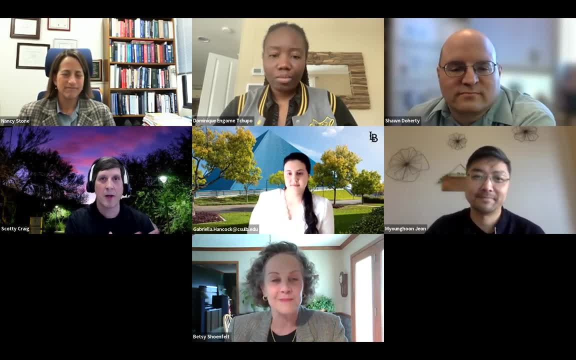 and you can apply those skills in whichever areas you want to go into, And sometimes you can stop and go into completely new areas, if that's what you're interested in. That's what Sean showed us, which is amazing. Okay, thank you. Rupa, I wish there was a way to make sure that we're using our skills the right way, But I've been trying to figure out ways for people to use their skills the right way, And it's really important to learn what we've learned and the skills we've learned. So I'm going to go back to that. 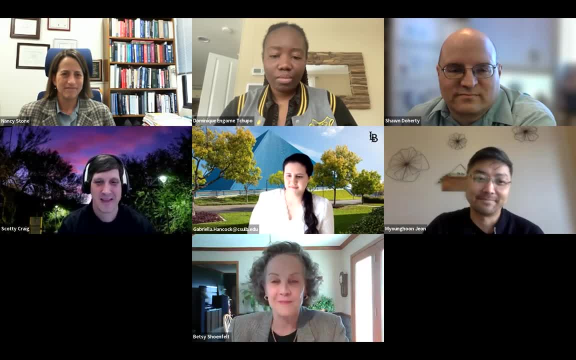 and I'm going to go back to my questions. I'll just share with you the questions as well. I'm going to go back to my questions. So I'm going to go back to my questions. had told me that it was okay to be quote, unquote, unfocused um, and that multiple interests can be. 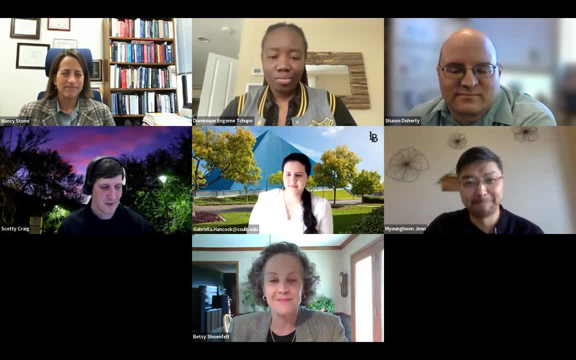 an asset, not only a distraction, and i also wish someone had told me that it's um, okay, or give me permission, but it's okay to let your personal experiences change the type of science you want to do. okay, sean, two quick things for me, and one of them- and you've heard it a little bit- 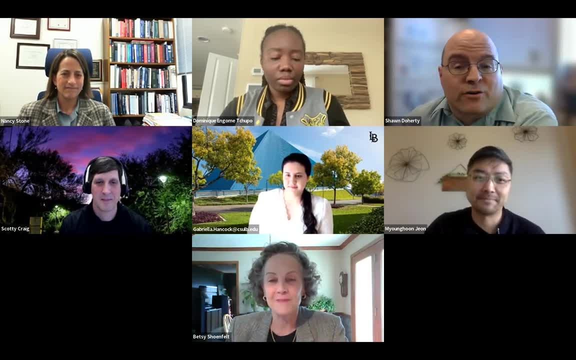 already. but, um, when you get to school, find a mentor- whether that is, you know, a teacher, and whether it's another student or a classman that's maybe a little bit above you, that can help kind of show you the ropes while you're in school. that helps a lot. you don't have to try and figure. 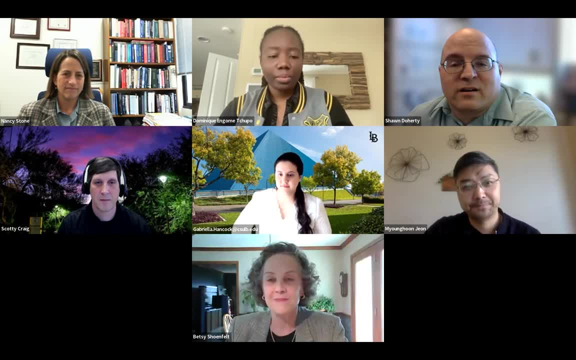 it out all on your own. there's a lot of people out there that are ready and willing to help. so you know, find a mentor and number two: one thing that i actually did kind of discover on my own that maybe will help is that, again, human factors. look to the 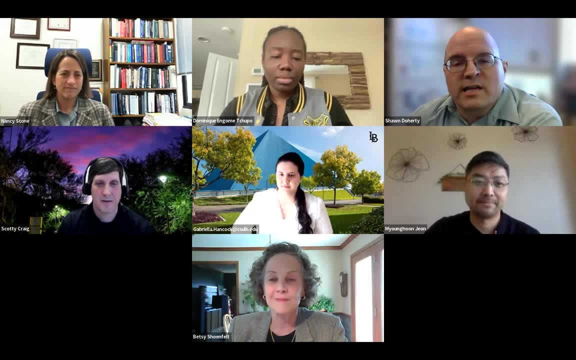 interface between people and equipment, which means that if you're working on a team with, you're oftentimes working on a team with a lot of other disciplines. so you might augment maybe your knowledge of human factors with some other areas like computer science or business, which will then